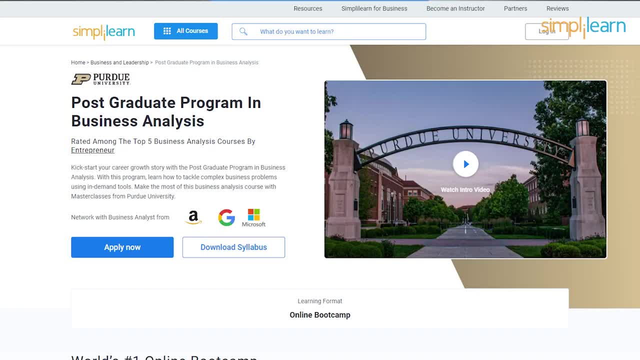 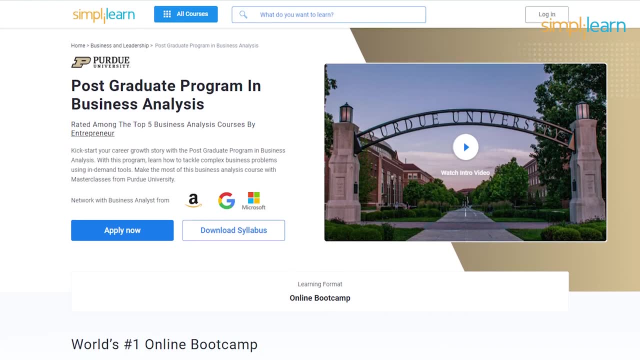 with business analytics by learning from the experts. then try giving a show to SimpliLearn's postgraduate program in business analysis that is from Purdue University and in collaboration with IBM. The course link is mentioned in the description below. If you are interested in learning more about SimpliLearn, you can click on the link in the. 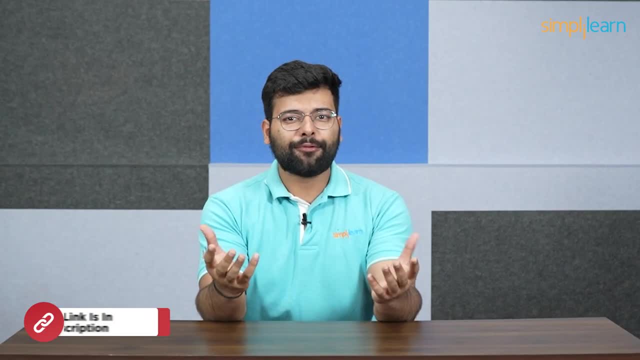 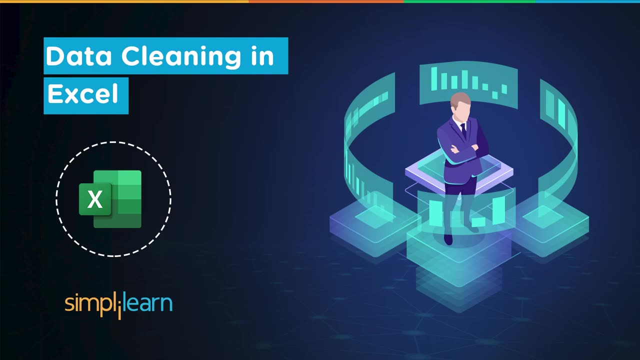 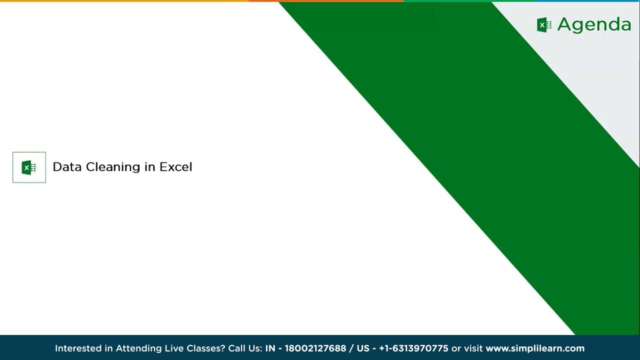 description box and you should navigate to the course page, where you can find a complete overview of the program being offered. Without further ado, over to our training experts. Hey everyone. so let's get started with data cleaning in Excel. So, without further ado, let's get connected to Excel, where we have the dataset that we need to 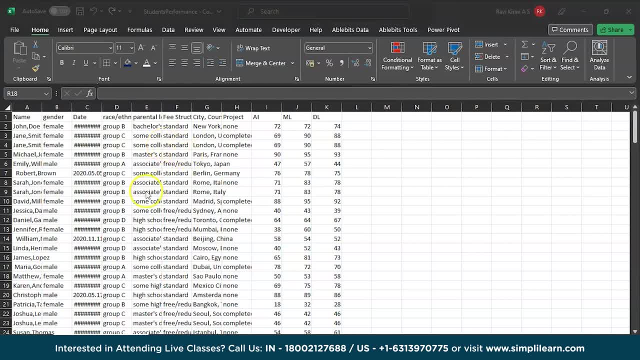 use to perform the data cleaning process. So right now on my screen you can see a simple dataset which has details of students. It has a calendar data, joining race or authenticity, parental level of education, peer country project and their scores and everything right. So we might have to perform. 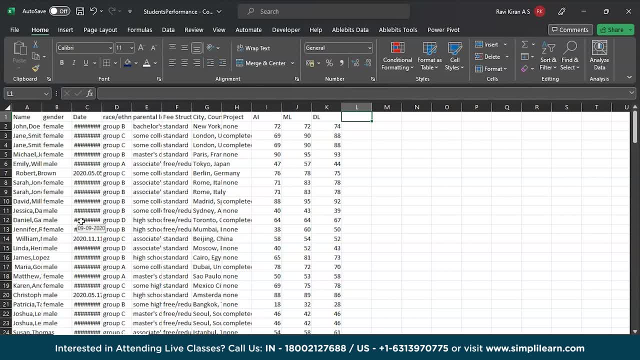 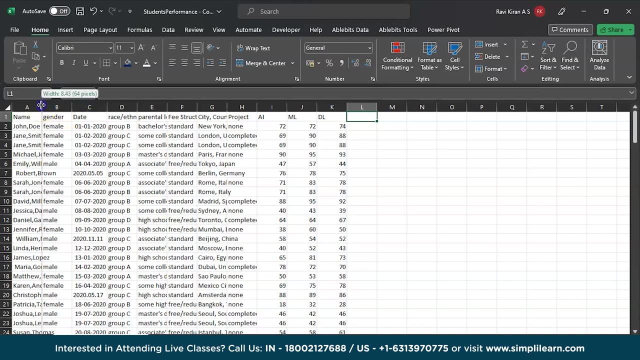 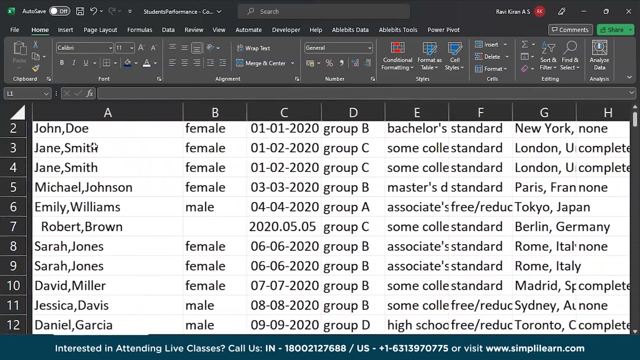 some data analysis operations and if you directly ingest this data onto data visualization tools or any of the analytical tools, you might have some discrepancies on the data, which might end up creating some discrepancies or abnormalities on your data report right. So, for example, if you can see this particular name section here, we have duplications in names. 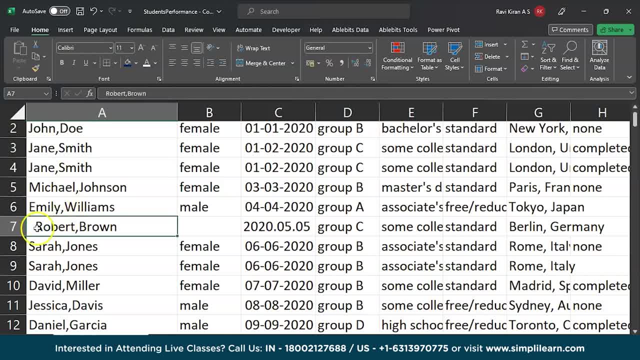 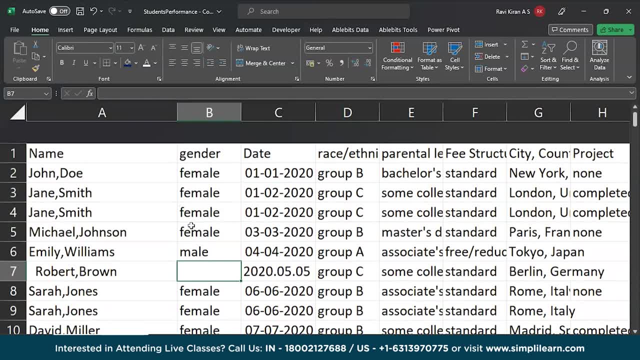 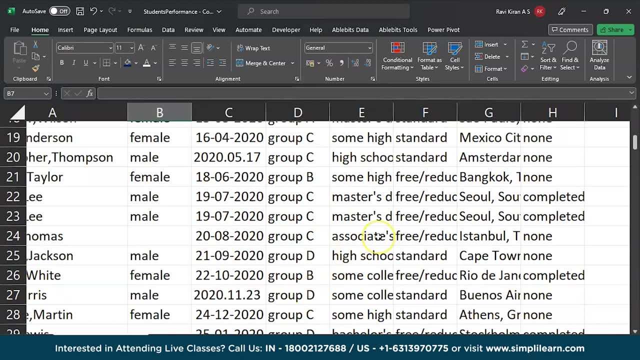 So we have Jane Smith entered for twice and in the seventh row you can see there are some blank spaces in the front of the name and you can also see there is no gender specified in this particular section, right, And if you also pay some attention to detail in the? okay, let's expand the. 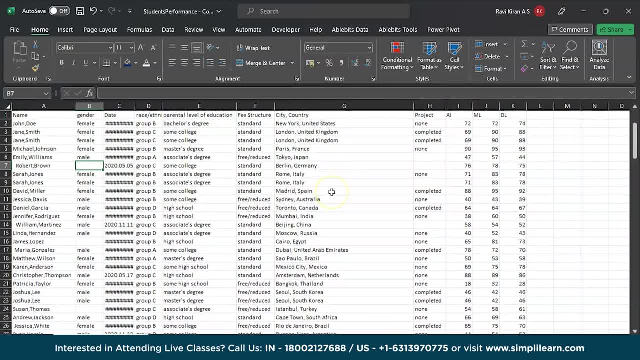 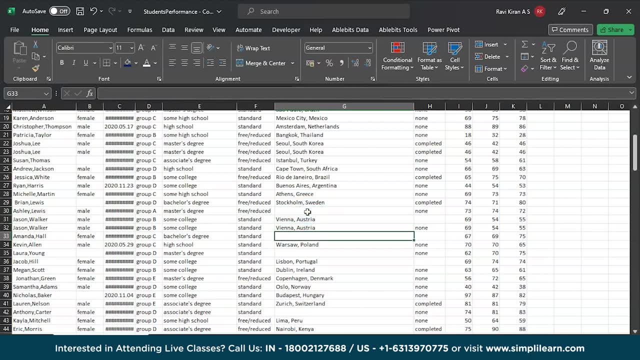 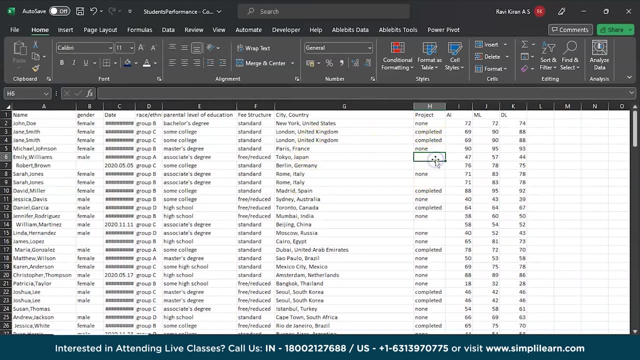 columns perfectly. first, yeah, into the column where we have country and city. there are countries and cities to every row, but in a few places we can see blank cells again and again. here in the section of project completed or not, you also have some blank spaces once again, right, And if you 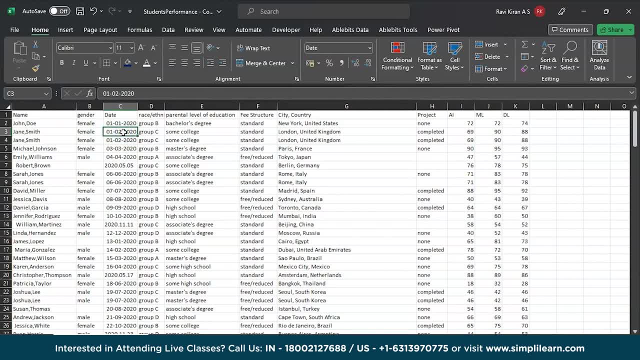 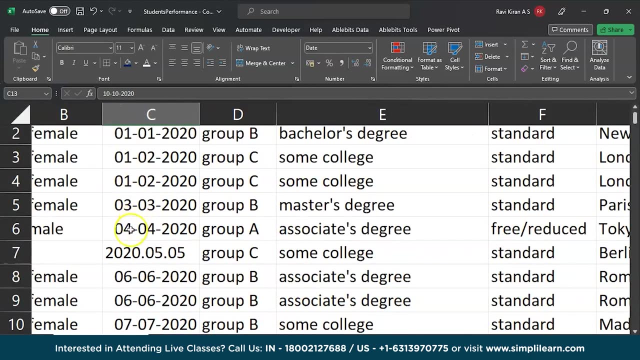 clearly check at the dates column. you have different kind of dates, right? I don't mean to say different data types. I need to say we have one single data type, that is, date, but the way the dates are written or represented is different. If you closely observe, we have 04 04 2020, separate by hyphen. In the next row you have 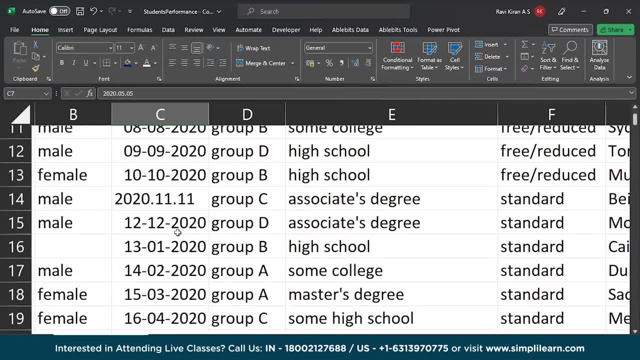 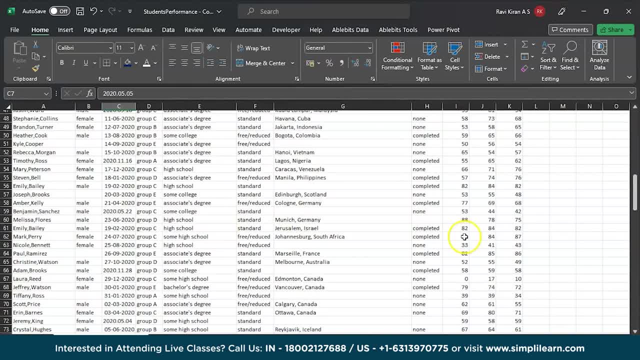 you can see that the date has been separated by- yeah, you know, dots and again, so slowly, somewhere we might have backslash right. So there are different ways of representing the date. So there are some anomalies in the data which you might have to clear. and again, if you want to add, 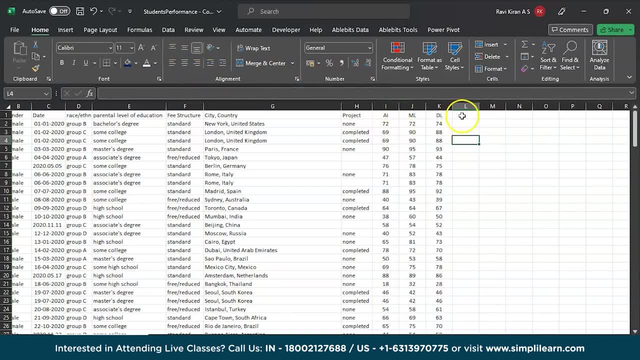 some formulae. let's say you have the student's course and you wanted to calculate the average score, right, let's say average. and if you also wanted to decide the you know class at which they have achieved their degree, right? so that can also be added here. So you can do that. and 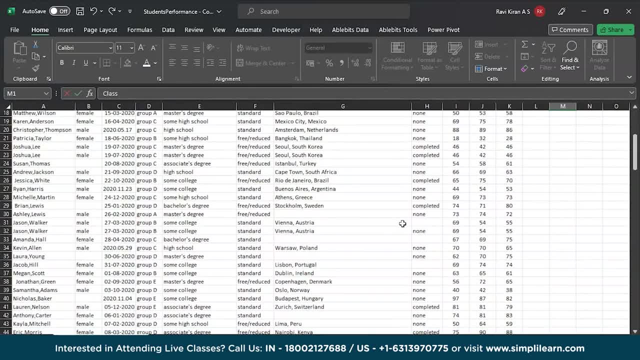 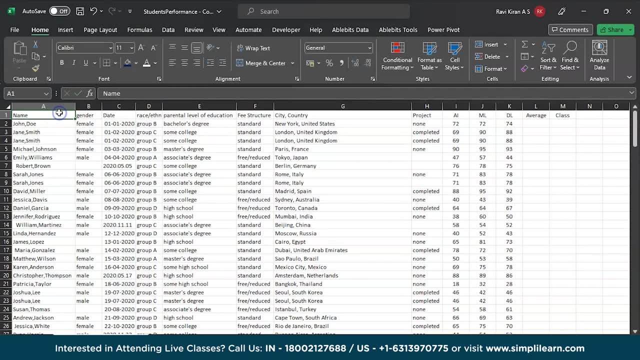 right. so these are the few problems that currently we have with our data which need to be sorted. So, before we get started, let's quickly create a copy of this data set right So that, as a bonus point, we will also do the same data cleaning process in power query, which can be a lot more easier. 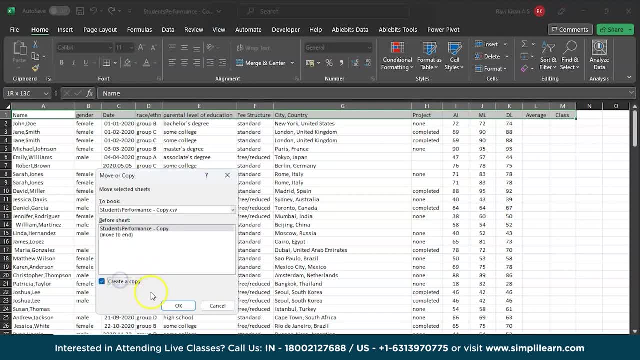 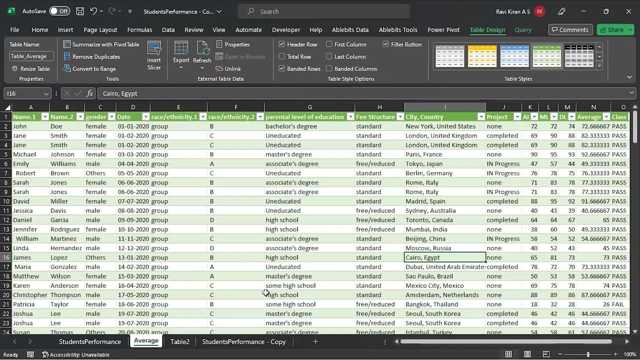 right, So let's quickly create a copy of this. So, before we get started with the power query, let's hear it from our learners about their success story. after graduating from the Post-Graduation Program in Business Analytics from Purdue University, I have always been passionate about learning new things and improving my teaching skills. 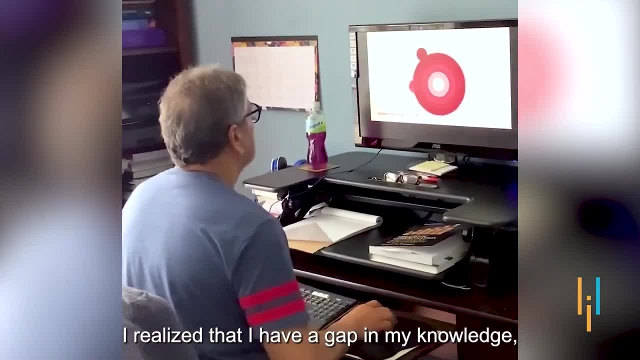 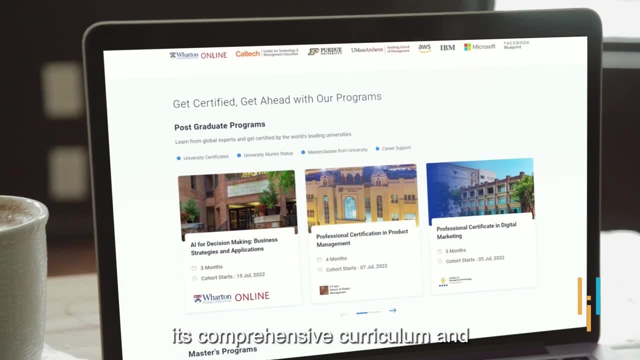 About five years ago, I realized that I have a gap in my knowledge and to fill the gap, I needed to upskill myself. I chose SimpliLearn as my upskilling partner because of its comprehensive curriculum and its connection with Purdue University. 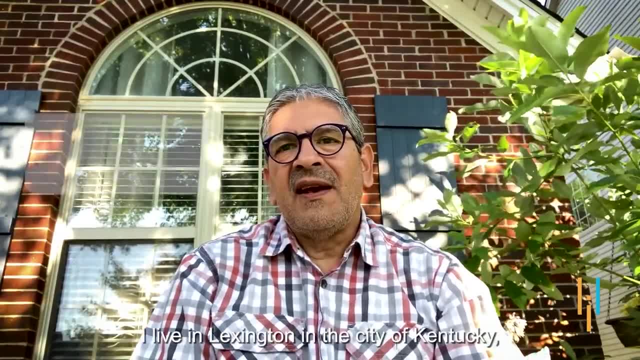 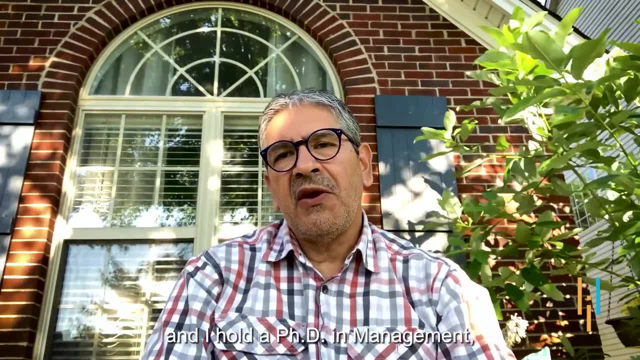 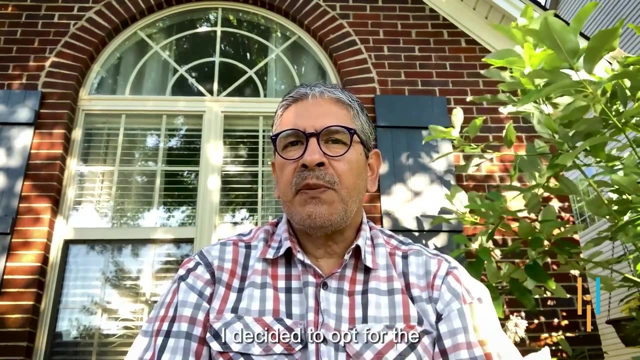 Hi, my name is Carlos Linares. I live in Lexington, in the city of Kentucky in the United States. I am an assistant professor at Midway University and I hold a PhD in Management, Human Resources and Leadership. I decided to opt for the Post-Graduation Program in Business Analytics from SimpliLearn, which 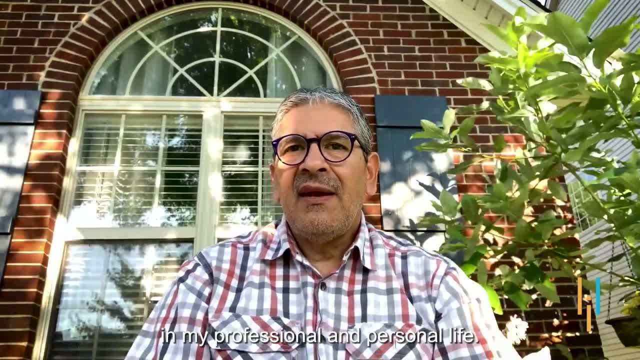 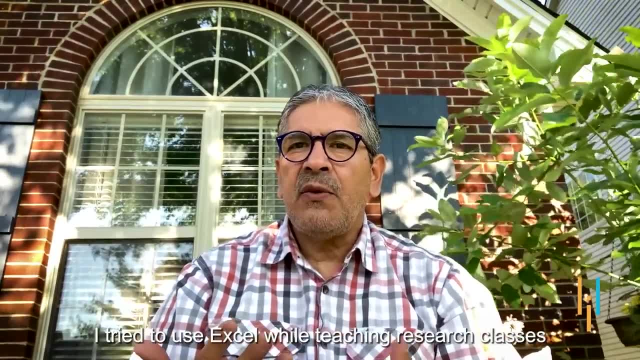 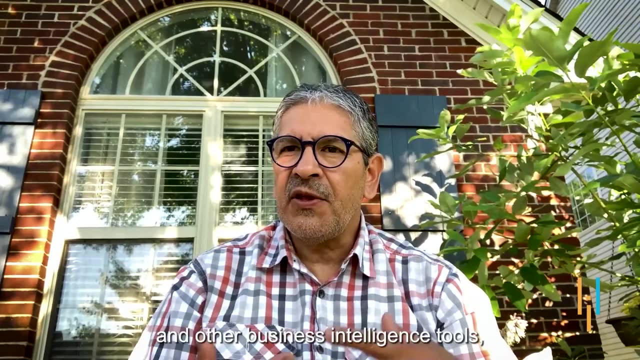 has helped me a lot in my professional and personal life. I have been teaching ever before I moved to the United States. I tried to use Excel while teaching research classes, but since I only had the basic knowledge about it and other business intelligence tools, it was very difficult for me at the beginning. 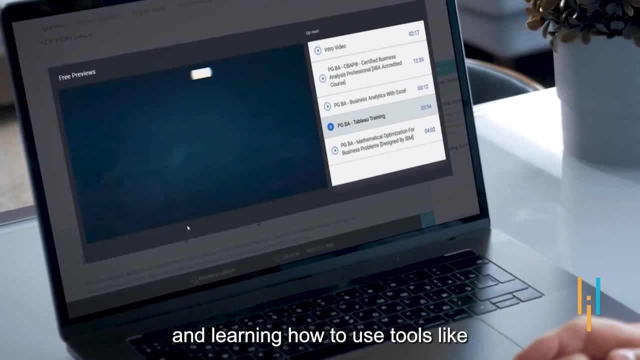 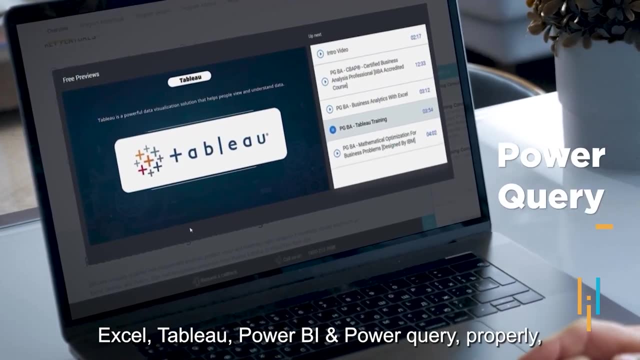 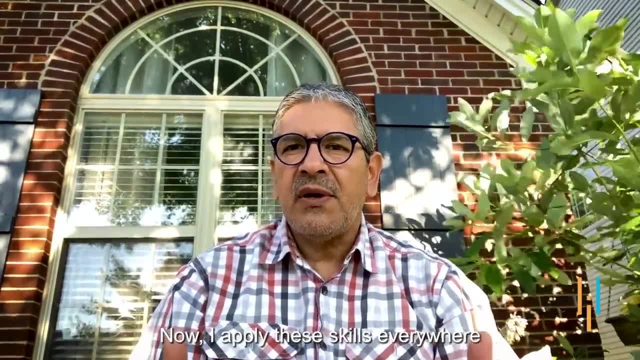 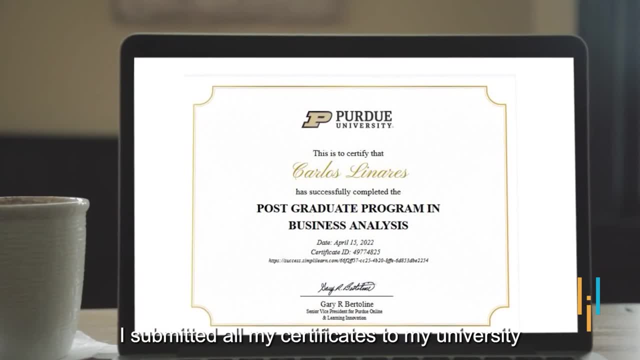 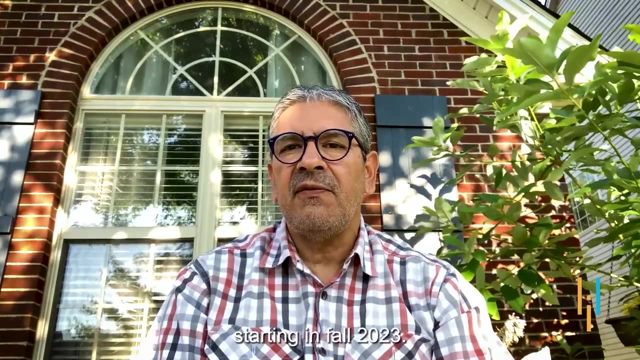 I have learned a lot. Now I apply these skills everywhere, which has also helped me a lot. in my yearly review, I submitted all my certificates to my university and, based on that, my university plans to develop a class focused on business analysis starting in Fall 2023.. 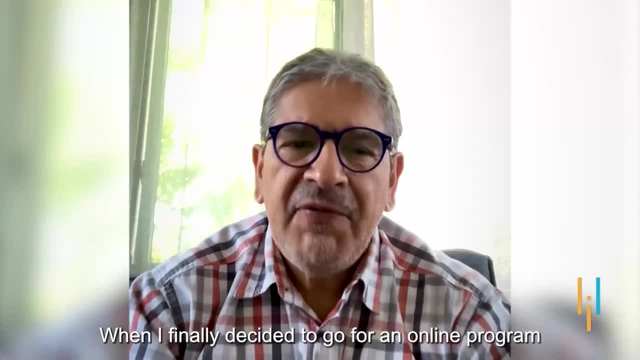 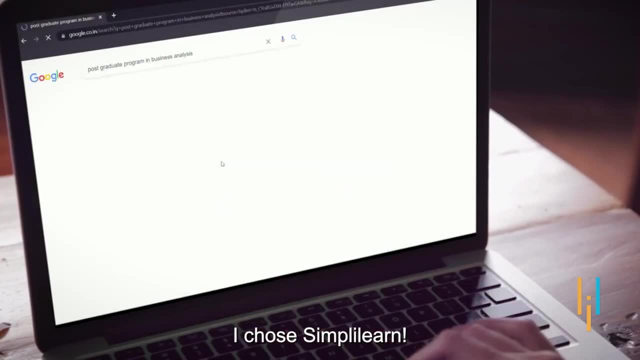 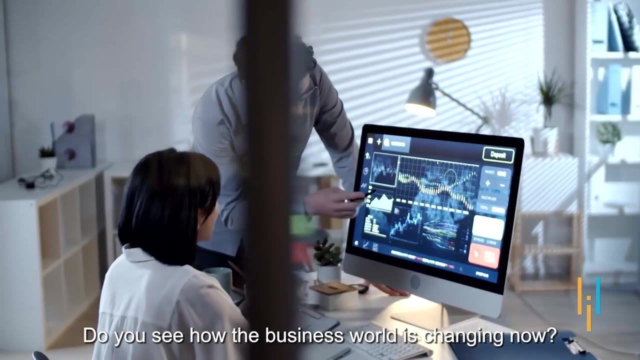 I am really excited When I finally decide to go for an online program. I research a lot. Finally I am excited. Finally I choose SimplyNerd And I must say it has been a wonderful experience. If you see how the business world is changing now and the skills you Telle is quite essential. 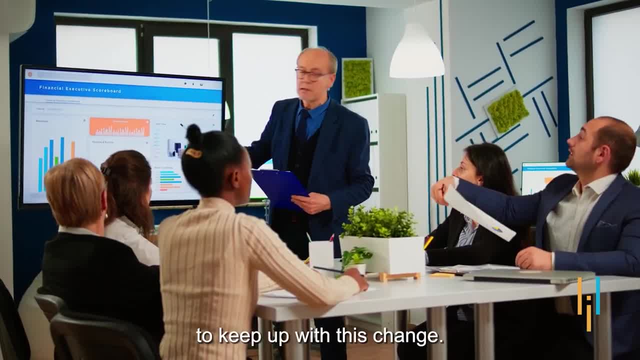 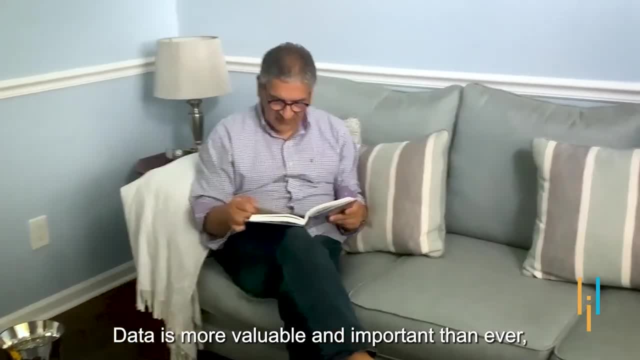 to keep up with the change. everything works on numbers. now, Data is more valuable and important than ever, So I encourage you to keep learning and keep growing. Now let's continue with Power Query. So I argue that it is more income-efficient to be an online experience than to be an online. 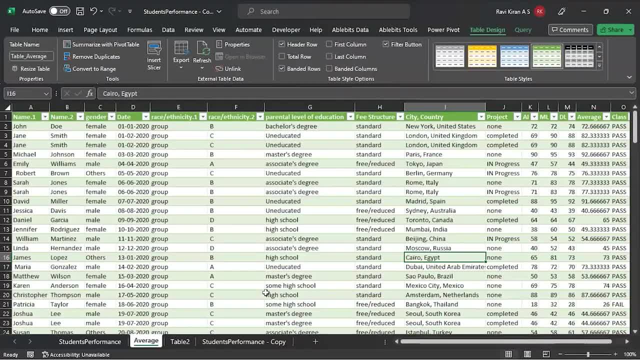 browser. And when you turn your accelerated learning to a virtual learning world- and maybe really in a virtual world, it will be hard to get full access to the services. It can get complicated, But why would you want to go for a virtual learning? 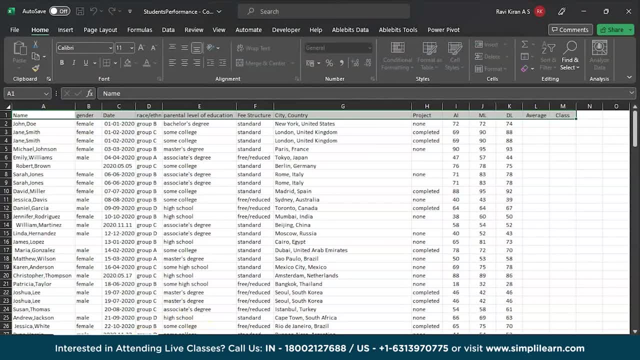 So why are we using Power Query again? So, whatever the data cleaning process that we are going to perform is good up to an extent, Because if you are dealing with some real-time data and if you are dealing with some data which almost changes every now and then, 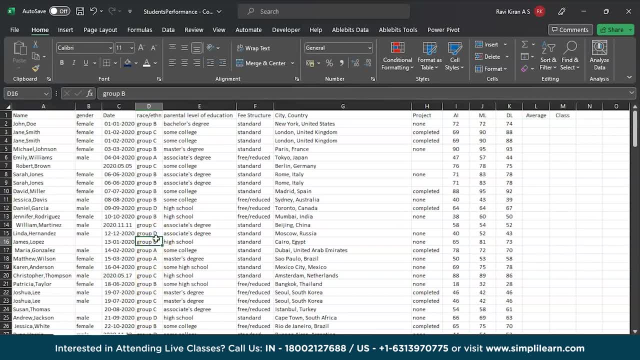 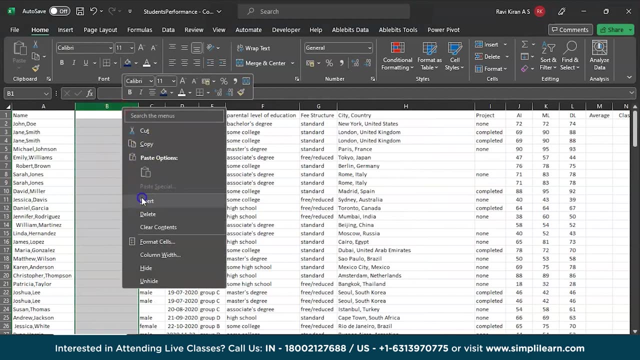 then the data cleaning process, which we are about to do, will be stagnated. Let's say, for an example, we have the first column as name column. As a requirement, you might have to, let's say, insert a new column here and another new column here. 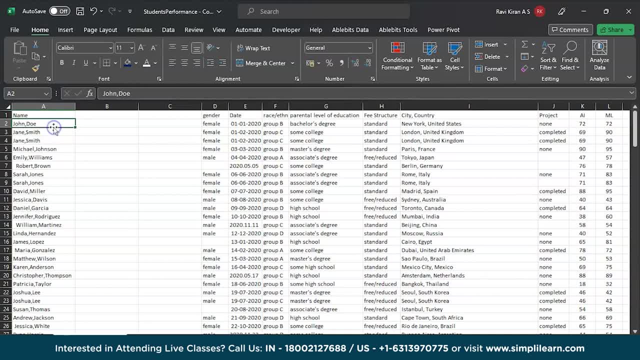 Let's say we have a requirement where your manager says that he wants first name and last name as separate right- First name and last name. So let's begin with the first stage right, So that you have a better understanding of what's the problem that we have with this routine way of. 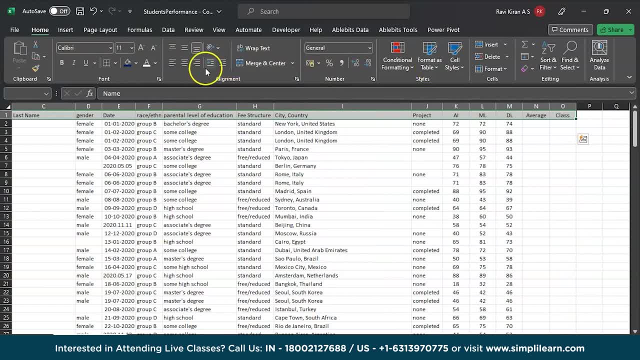 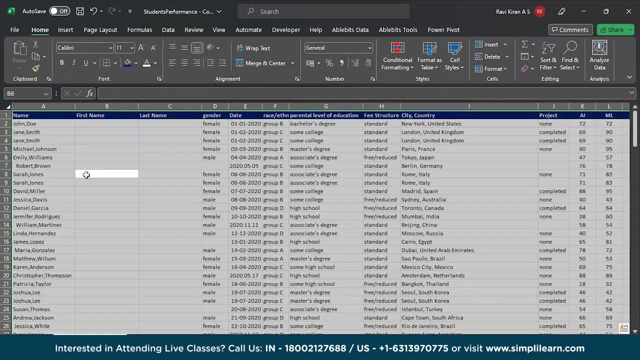 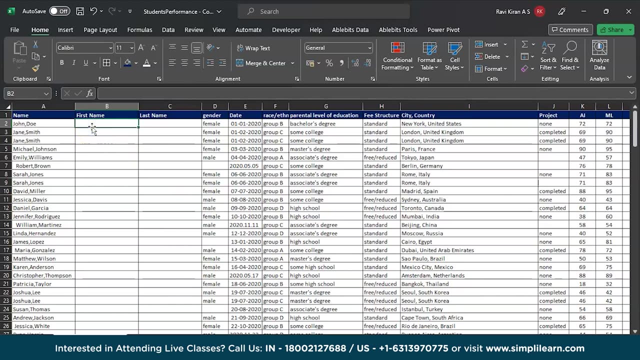 uh, cleaning our data, right. So, firstly, let us make our data look aesthetically correct. Let's add some boundaries and all the things that make it a little more better looking, right? So the first one: let's try to split the first name and last name, right? 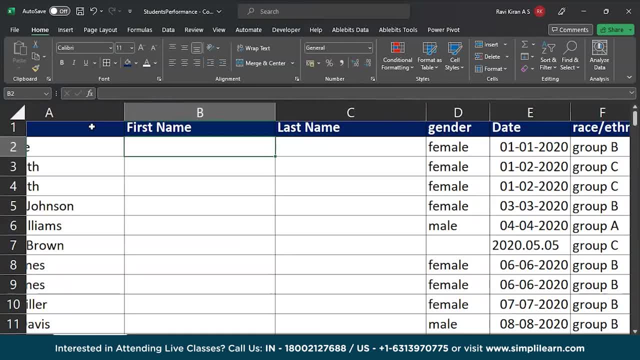 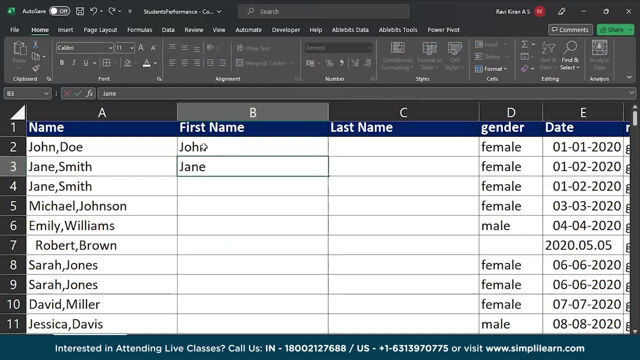 So here you can see, the first name is John Doe, right? So I'll be writing J-O-H-N- Hector, and J-A-N-E, right? So when I was about to type the first name, you can see something got highlighted, right? 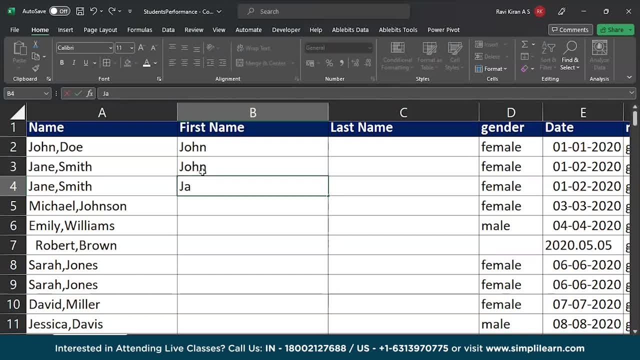 J-O-H-N And again if I write Jane once again and Michael right. So it is able to predict that something is about to be coming out right. Excel is able to predict that there is something in user's mind. 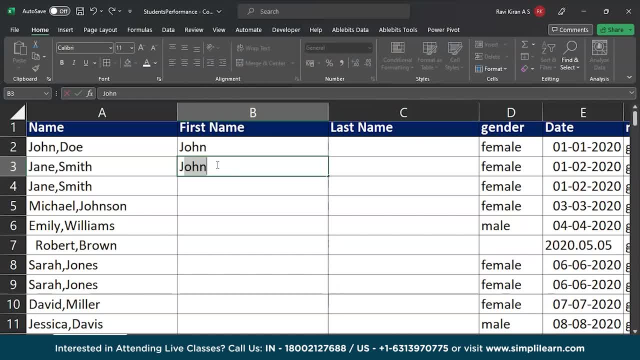 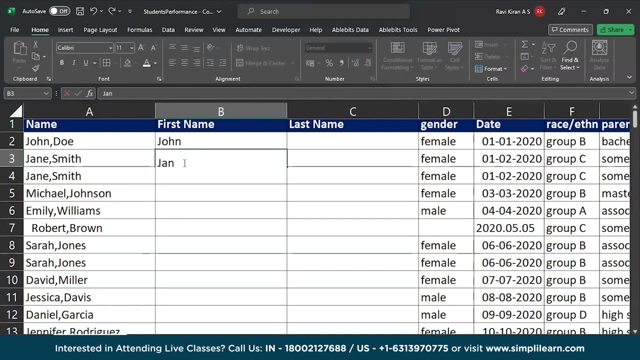 So maybe, if it's that what I think right, You can see it automatically suggested me. So it is trying to understand what you want to do. So that particular feature of Excel is called as flash fill. right Right now you have entered this first name and second name, right? 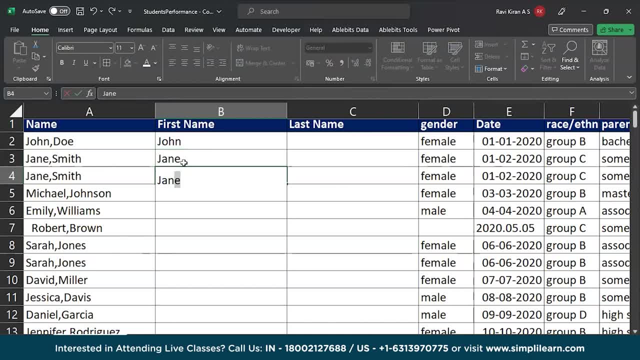 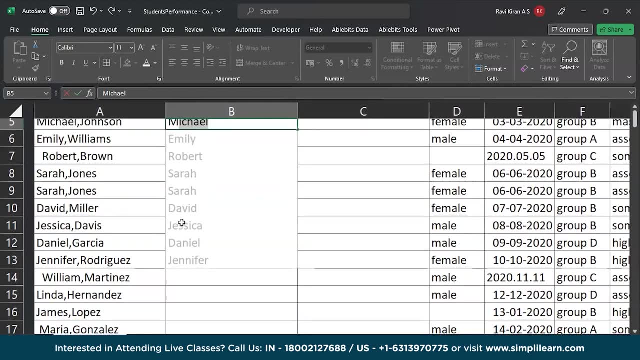 You have entered first names and here Jane once again, And let's try, Michael, And see if I minimize the screen. you can see it is showing the entire data set, right, It is splitting the first name of column A from the entire data set. 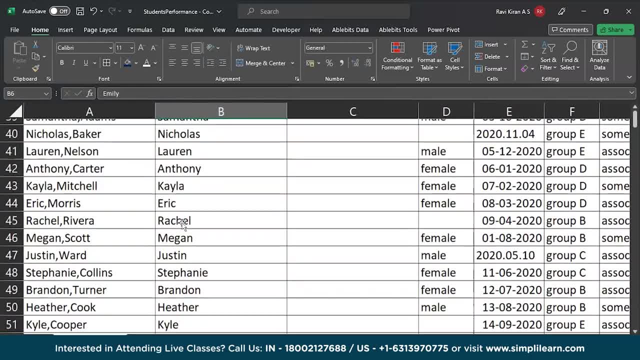 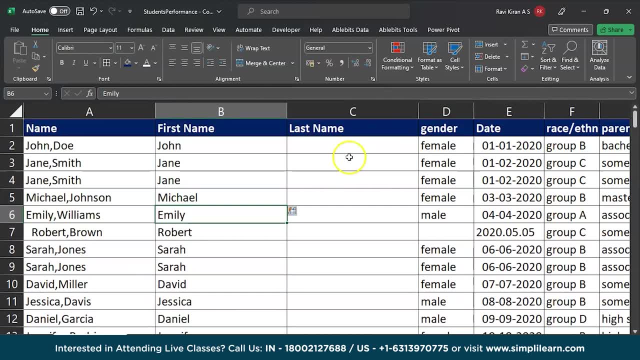 Just press enter and you can see it has entered all the first names until the last row right, Just within one single press of an enter. So that particular feature of Excel is known as flash fill in Excel. Now let us try the flash fill once again by adding the second names of each and every student in the data set. 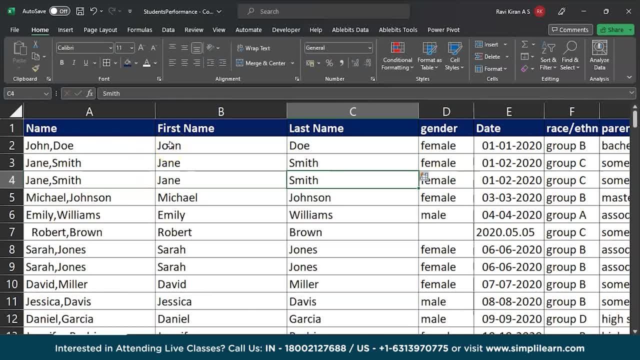 Press enter. There you go. Now, what was the problem? right? Flash fill works if the data is stagnant. It is a very fast and quickest way to split data, And you can also. okay, let's try another different way as well to split the data. 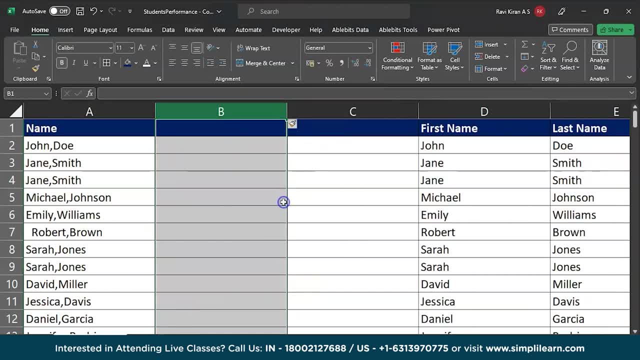 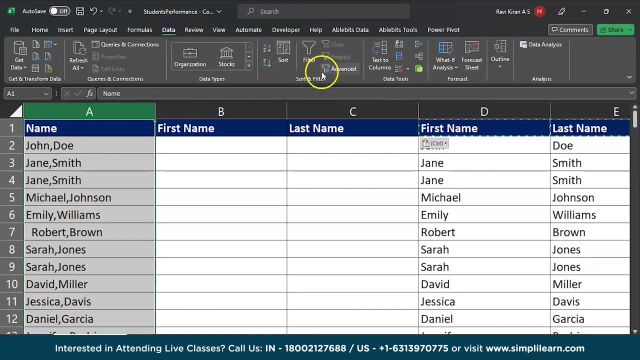 I am going to insert two more columns with same name: First name and last name. right Now, let's click on the column, Select the column and go to data, And here we will have an option called as text to columns. Yes, 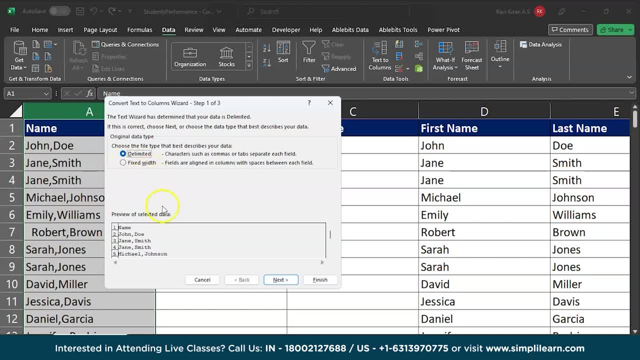 So here our data is delimited with comma. So go to next. We have selected the delimited option over here, Fixed width and delimited. Let's also check the fixed width one first. Let's go with delimited one right. So here let's select comma, because we have comma, and click on finish. 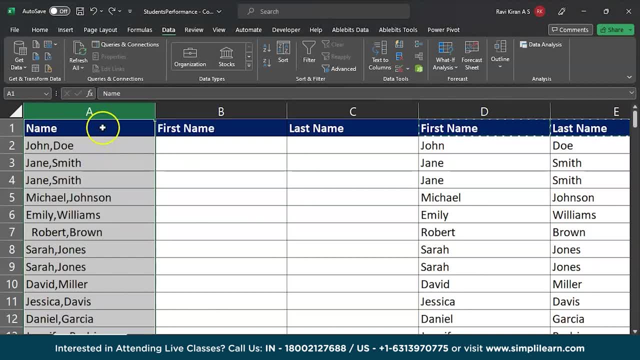 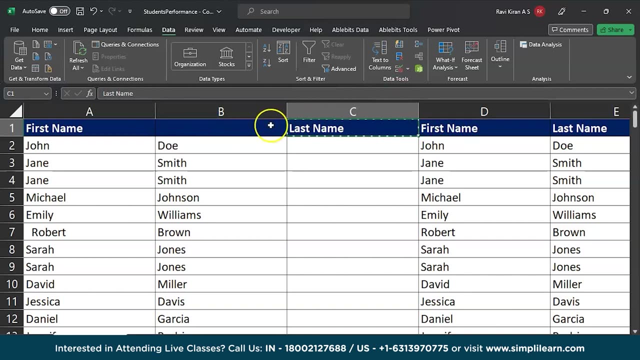 Okay, So it is splitting in the same row itself. It is also okay, Not a big problem. So it has split the first name and last name automatically, right? So let's have it over here. Last name Here. 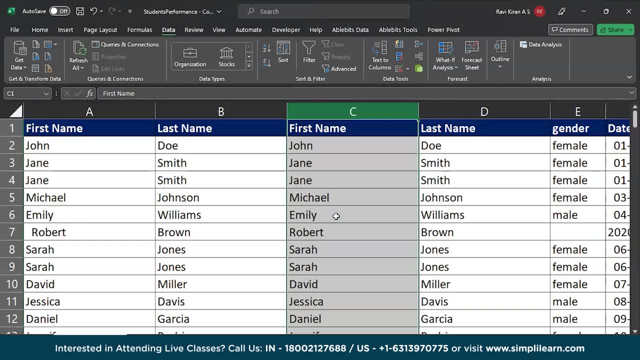 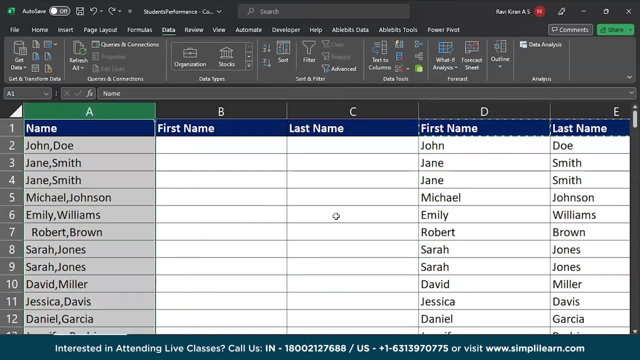 And since we don't need this particular Column, we can delete it, right? So here you can see. we have first name and last name. okay, If I undo all the process, right? Okay, What I can do is insert copy cells here. 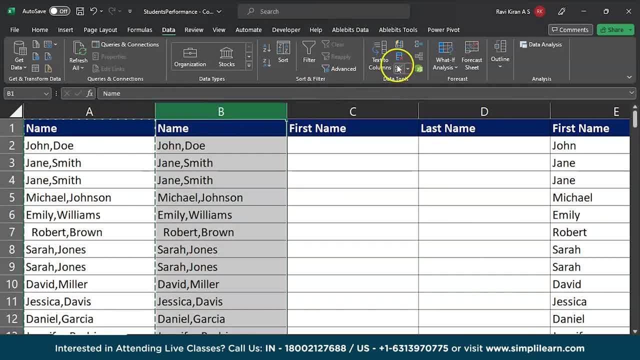 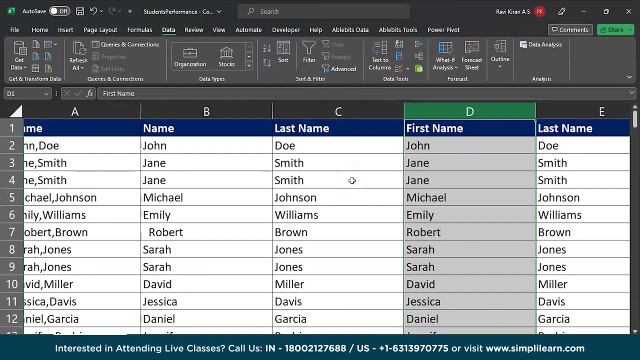 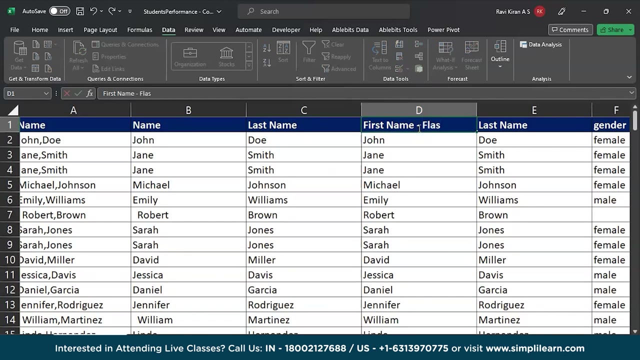 Now split this particular thing into columns so that I do have the original column. as it is right, I have it over here, So I'll delete this column. Now we have both ways. First is the flash fill one. This particular one is- let me name it as flash. 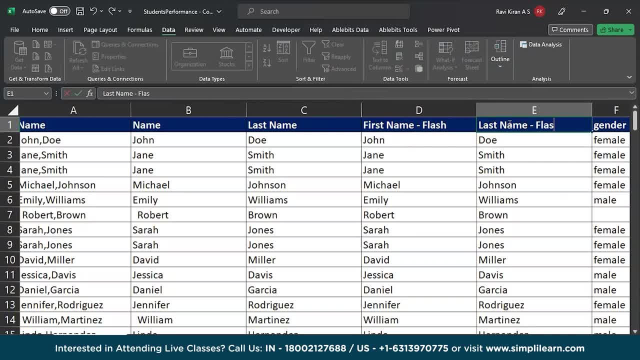 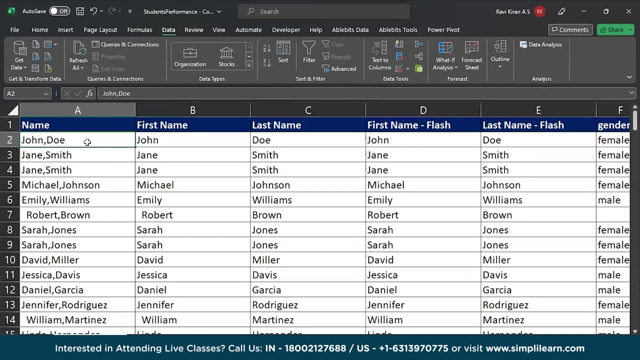 And this one has flash as well. right, So that we have two different methods, where data got split from first name to last name, right? So what's the catch? Now let me change the name. Okay, So let me change the name to the original cell. 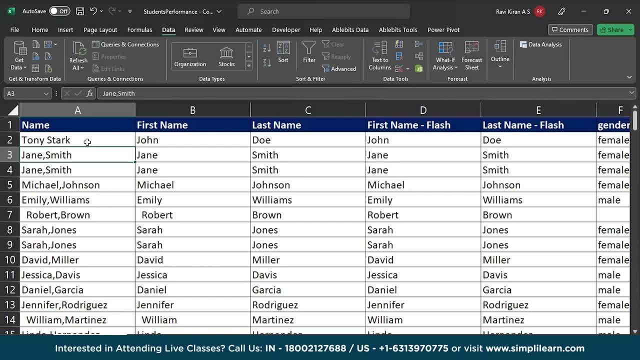 Let me name it as Tony Stark. Now you can see we used split text to columns in the first place, That is, this particular one, and the flash fill in the next option. But when the data got changed here it is not representing in the same way, right? 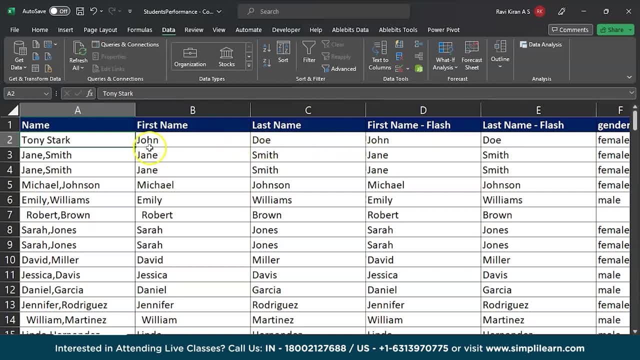 It's not catching the new entry into the cell or original cell. So that is the problem. So that is the problem with this particular one. We'll also solve it through Power Query. So first step of cleaning text is the split to columns that we did. 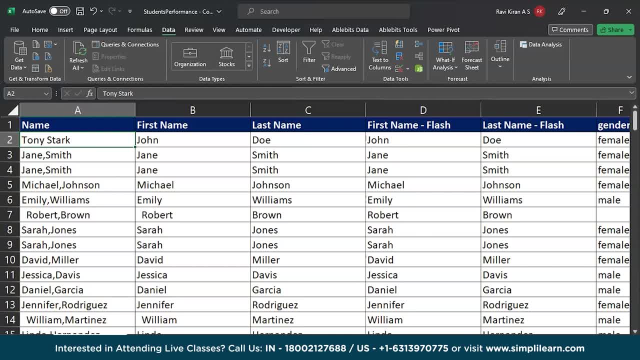 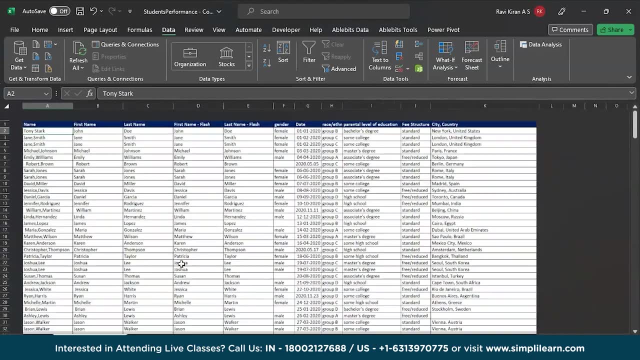 And let's also check on a few more anomalies which we had, That is, blank spaces, formulas, etc. We'll also check that one. So so far we finished with text to columns and flash fill. Now let's minimize the cell size again back to normal right. 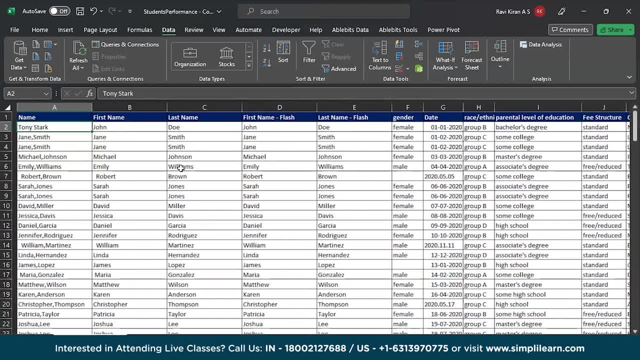 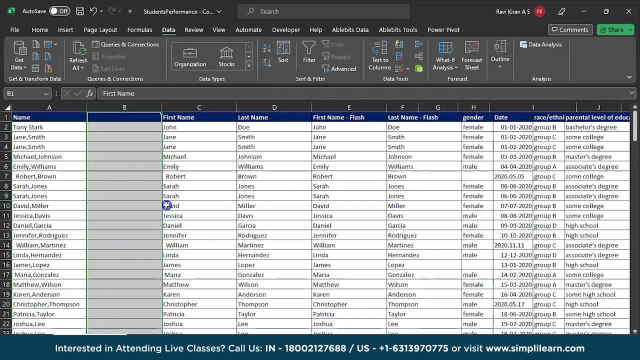 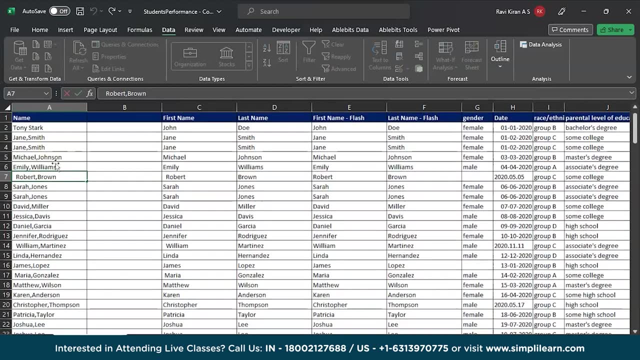 And now let's try to, let's say, remove this. Or okay, let's try to insert a new column here. And since we found that a few of the cells had extra spaces over here, let's try to remove those spaces by using the formula. let's say: 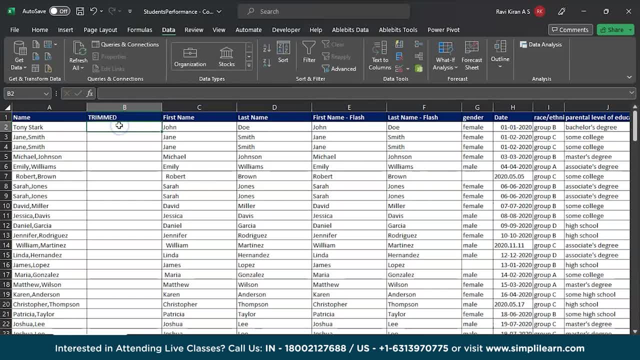 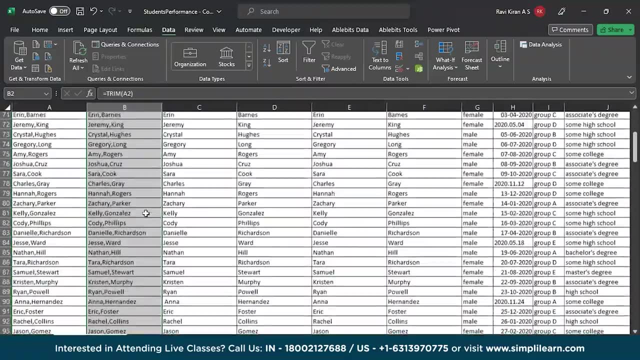 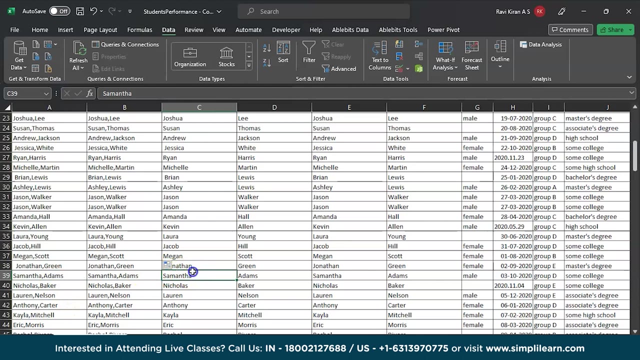 trimmed equals to trim function And select Address: Enter So you can extend the same formula throughout all the rows. And now you can see all the extra blank spaces are being removed out right And you can see previously when we used the flash fill right. 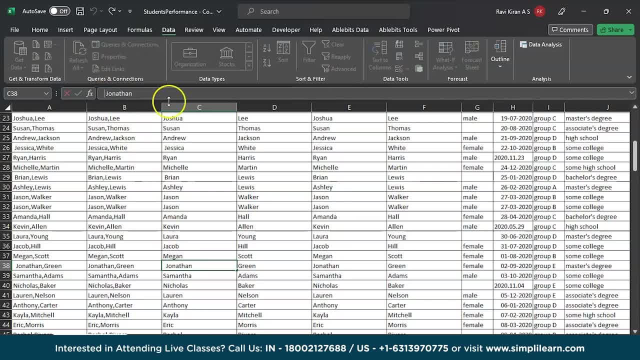 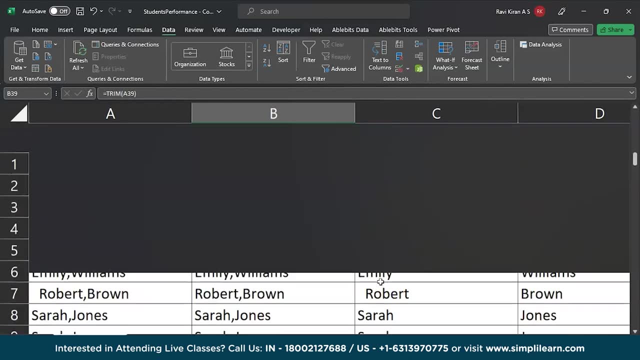 So it is having extra spaces, right, You can see it retained the extra spaces which we didn't need it. So if I expand the sheet, you can see the extra blank spaces. what we had in the original cell got retained in the resultant cell as well, right? 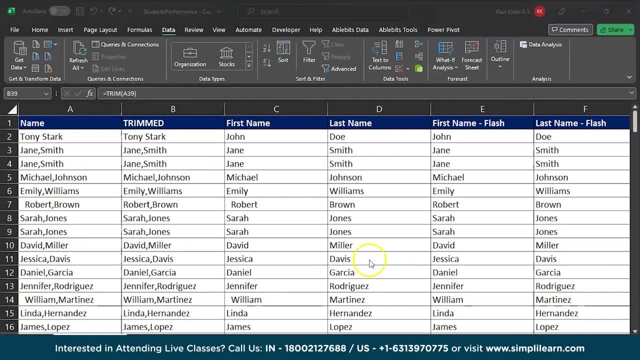 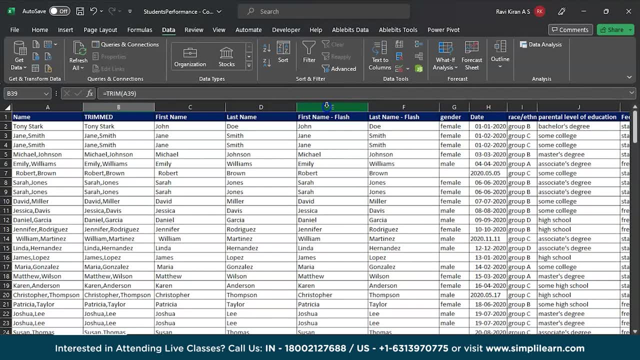 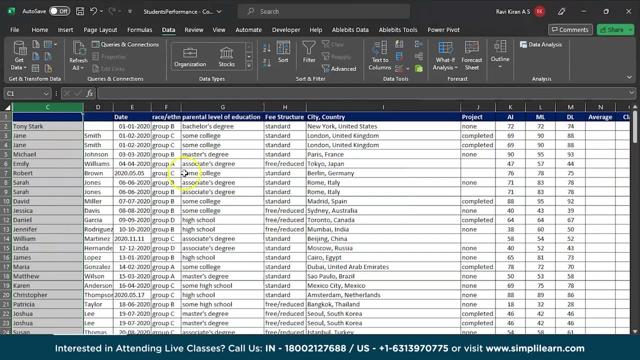 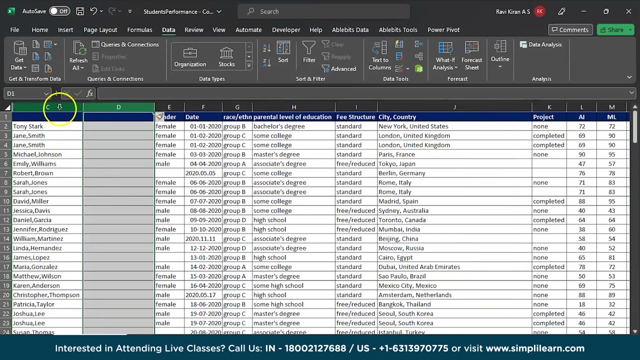 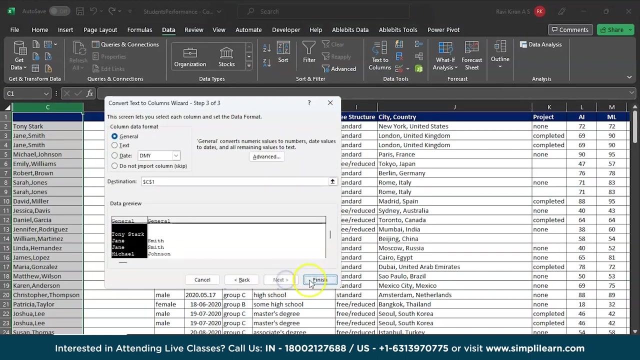 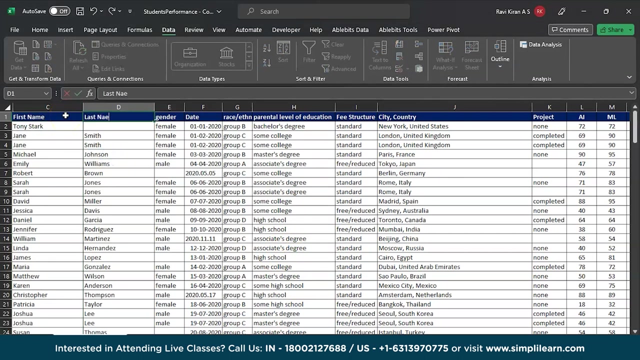 Let's try to avoid that. So let's try to minimize the cells back to the original size, And now you can conduct the same operation where you can, you know, kind of eliminate all the unnecessary cells. Now we have the first name and the last name. 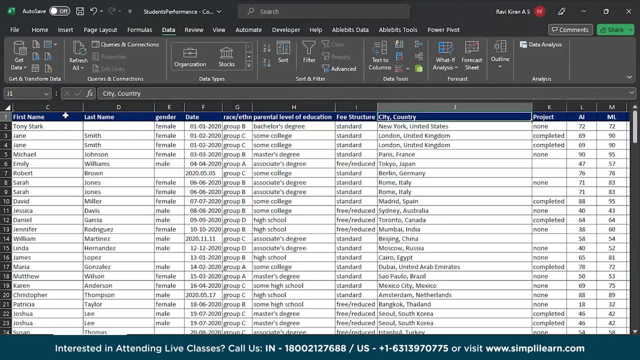 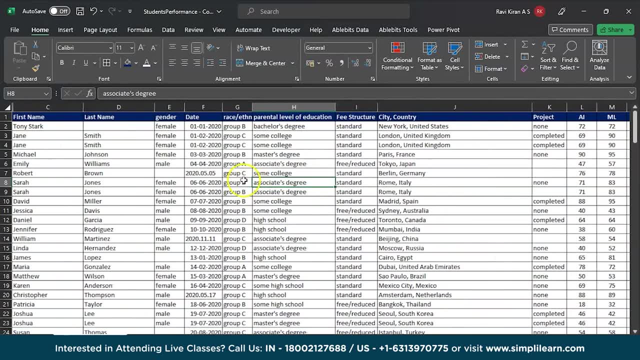 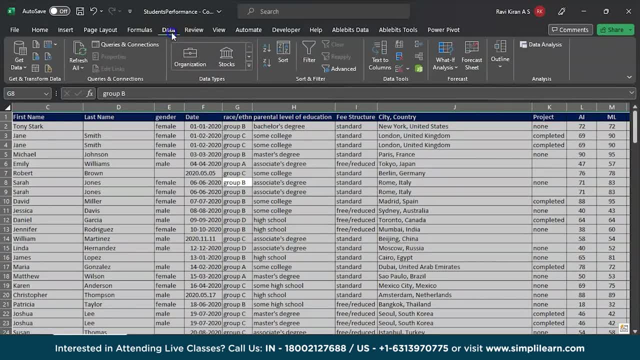 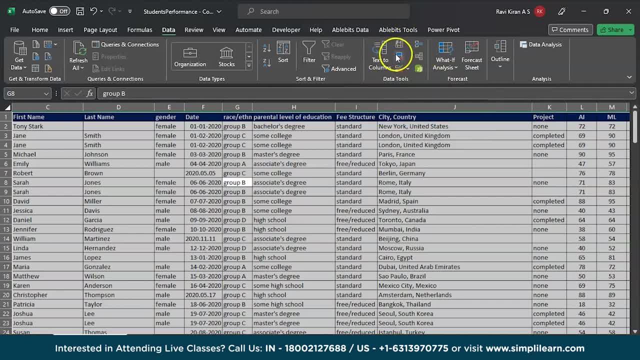 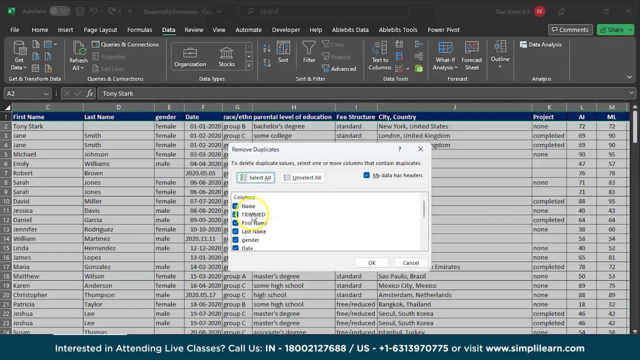 group and in the data tools group, select this particular icon which says remove duplicates. now it'll ask you based on what parameter? so let's give it one single parameter. so let's uncheck all the select, all the options, give it to one single primary key kind of thing. so here we have. 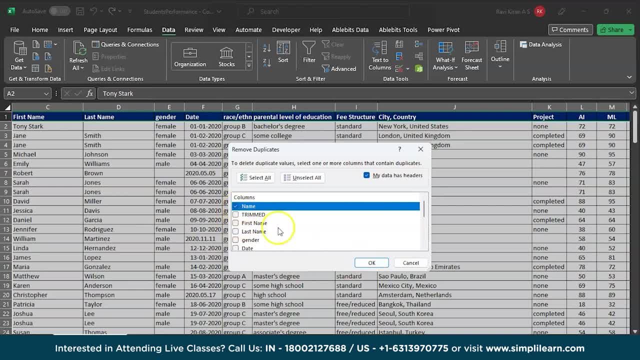 name, so click on that, or you can also give it as the first name anything which is which is unique for that particular instance, and since we don't have a unique primary key, i believe we have unique students here, so i give you the option called first name and based on first name. 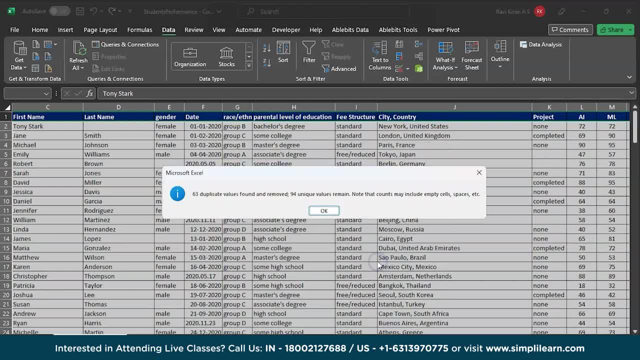 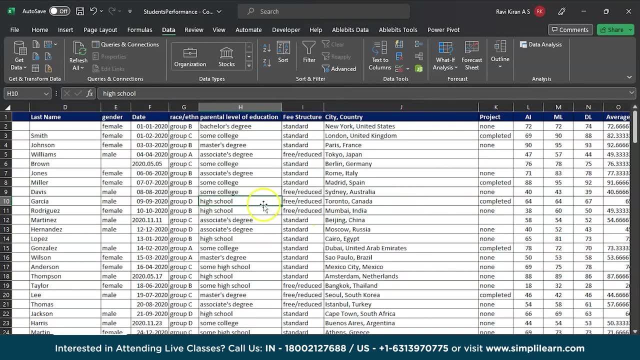 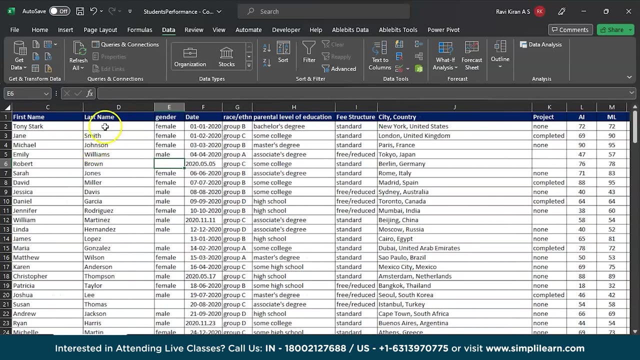 keep all the unique identities. press on, ok, okay. so so far we are good with the data, and now we have the blank spaces right and let's try to replace the gender column first, so wherever we have a blank spaces, then there you can eliminate the. uh, you know you can keep the space filled with as others. okay, let's try to do it. 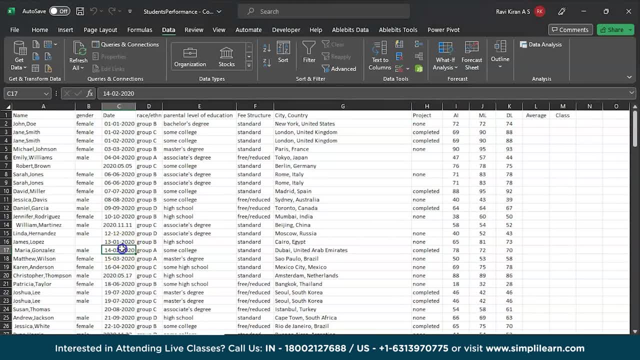 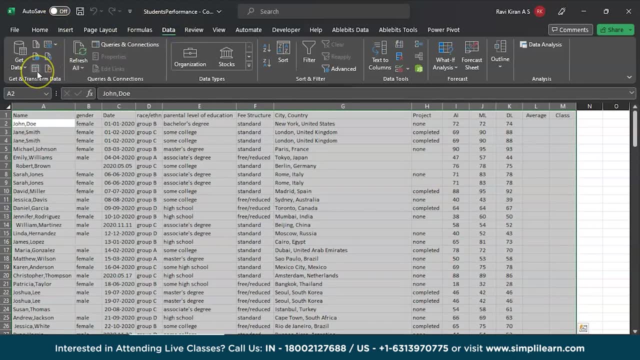 let's go to the original sheet before we perform any of the operations and here select the entire range. go to data tab and click on the option from table range so it has automatically selected the range, and click on my table has header so that your power query window knows that the first 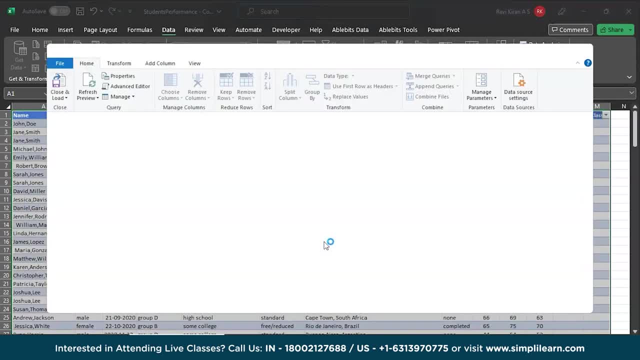 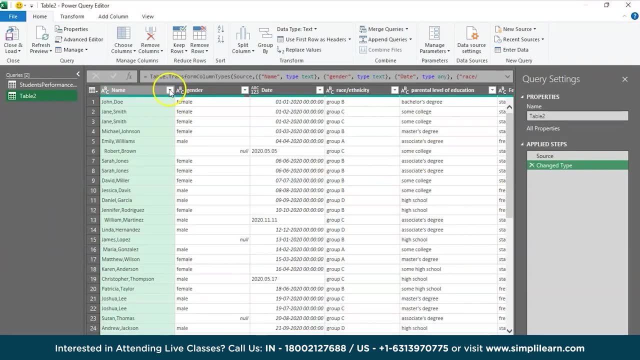 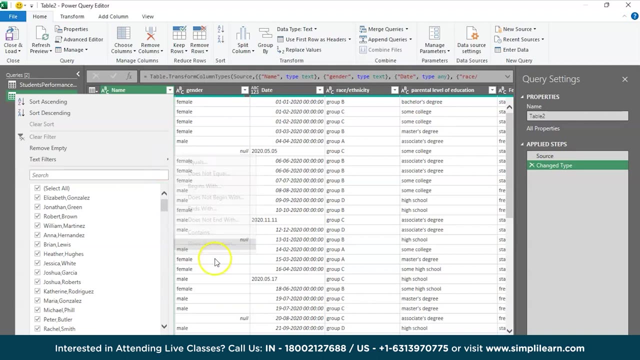 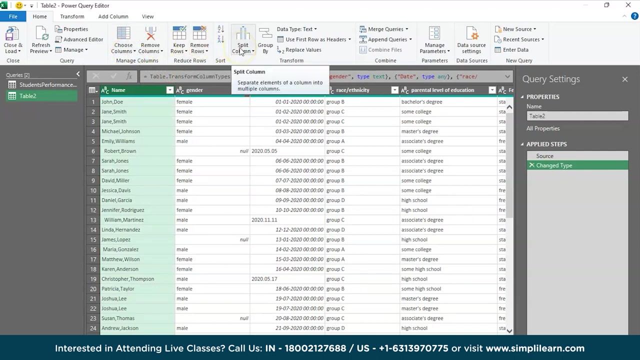 row is the headers. right click on. ok, and now we are on the power player. you know, power query editor opens application podobus. so uh, uh, first time we built it, i made it. it's a separate box in my library from your computer. so here you have the option to split the. 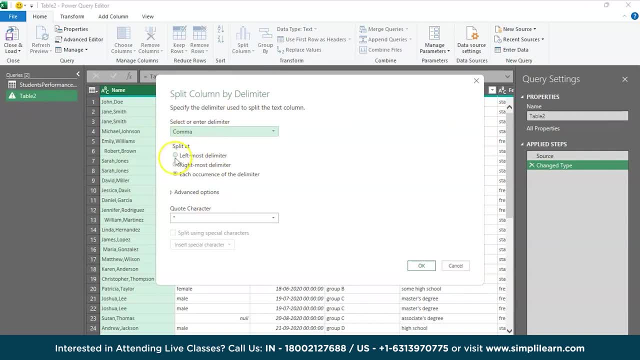 column into first name and the second name by d limiter and our delimiter is comma, so delimiters, right? so your name can be John Doe and another name which is separated by two commas here, right? so we don't want that to be happening. so if we have three instances or more than two instances, 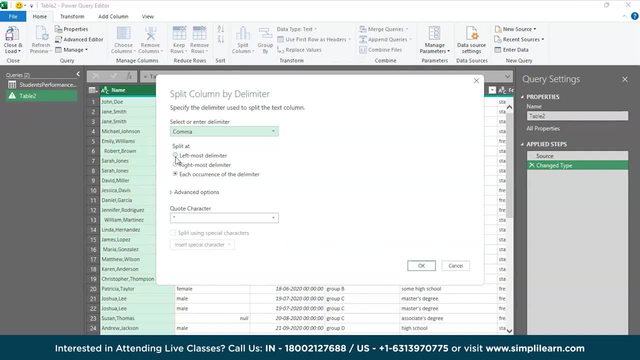 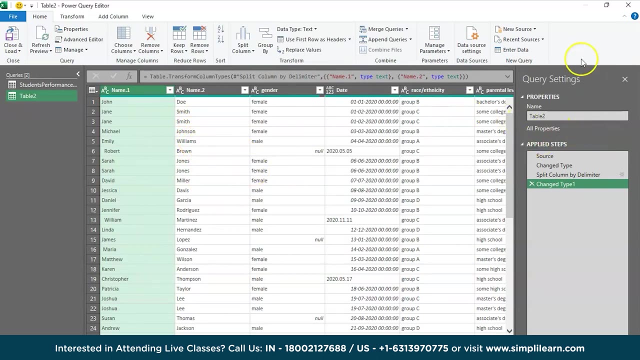 of comma, it will create two to three- uh, you know columns. so we don't want that. so let's provide left to most delimiter. so once if it has occurred, then it's enough. right now we have the first name and second name successfully registered and on the right side you can see we have query settings tab. 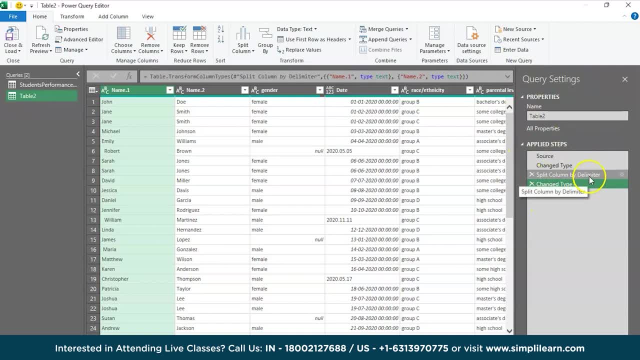 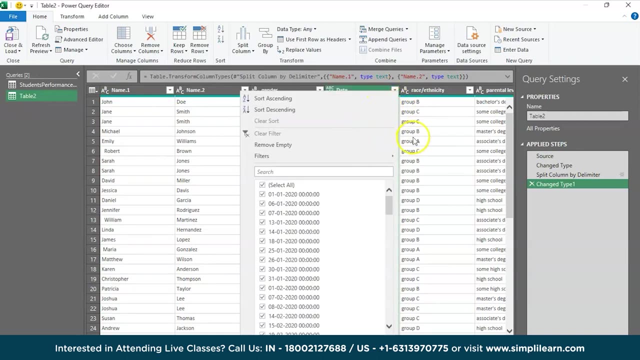 and applied steps tab. right here you can see each and every action. what we are doing is being registered so that if you want to create or if you want to run the same operation once again, you can just click on that and it will apply it. now, here we have different, different dates, right? so let's 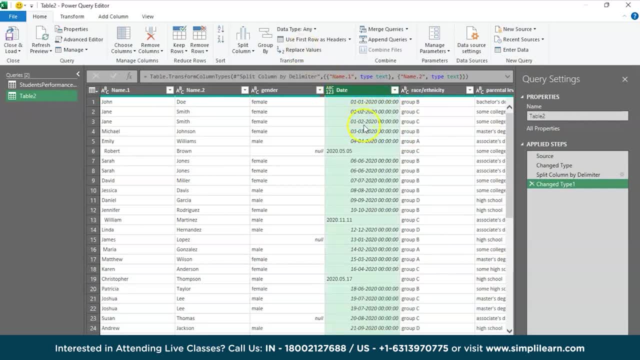 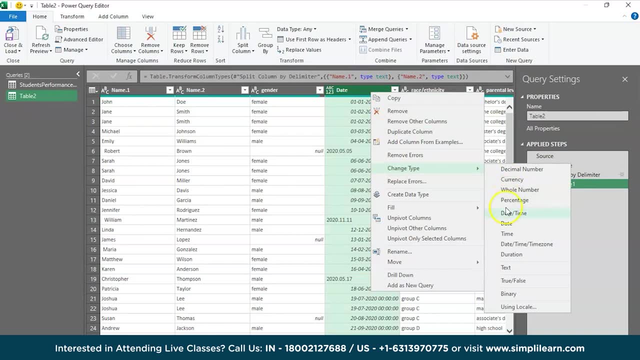 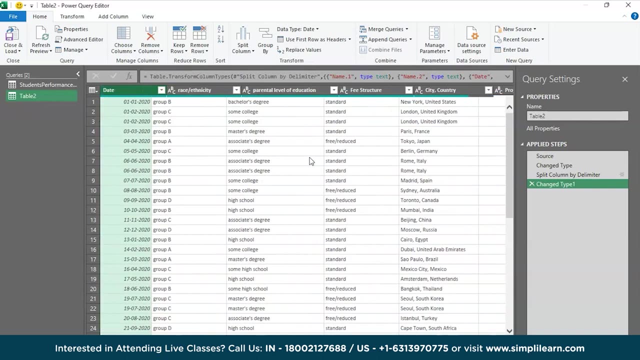 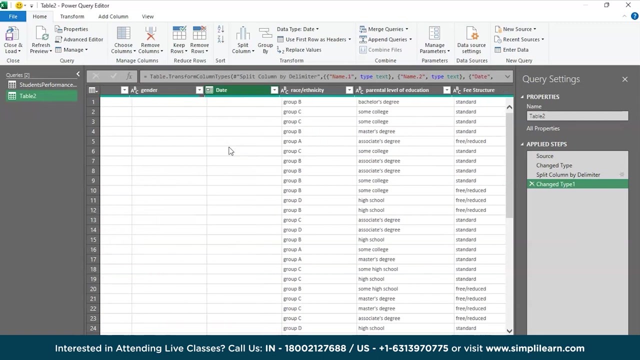 try to format the dates as well into one single single date format. right click and here you can see change type option. so here you can click on date so that all the formats run into one single type of format. right, and here we have some null elements registered. so let's okay. let's go back to gender column and here let's try to replace: 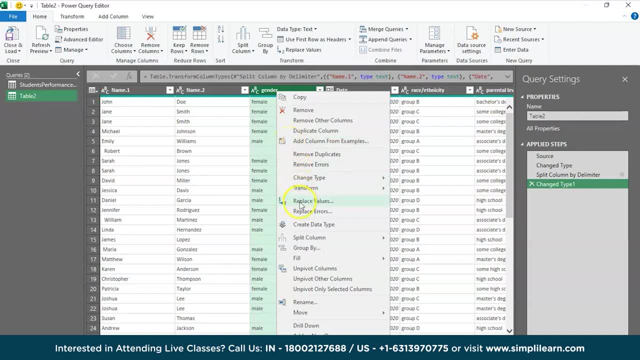 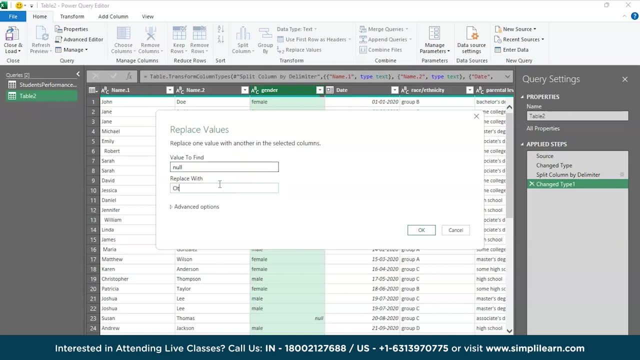 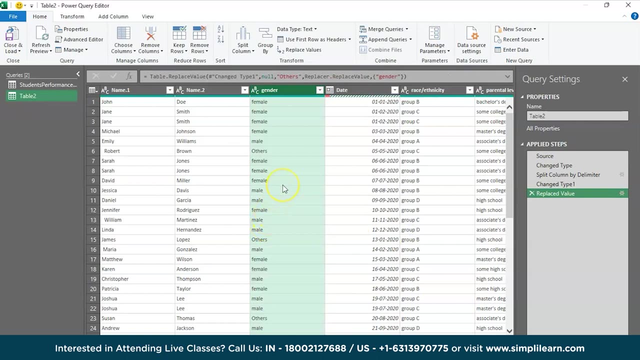 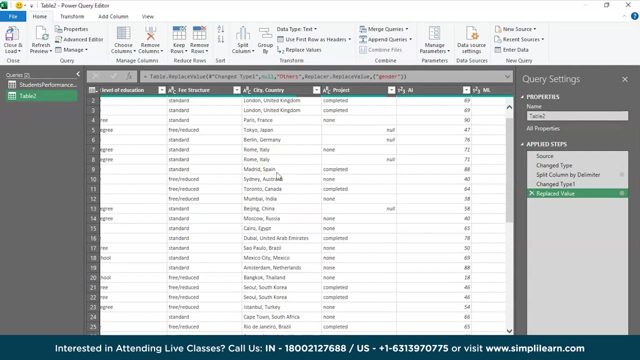 all the null values with others. so click on the replace values and here type in small case or lower case and replace with others. press ok. so wherever it finds null entry it will replace it as others. now coming back to the project column: and yeah, the country and the city column right. so here as well, so you can see. 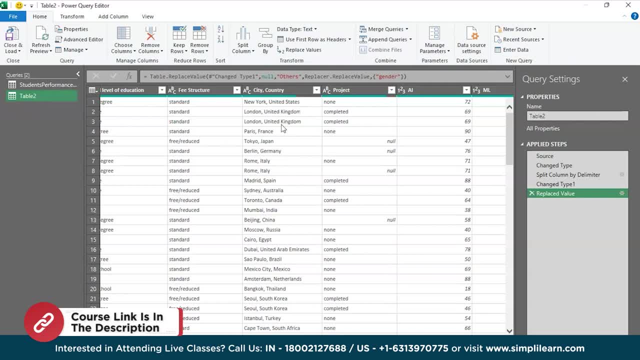 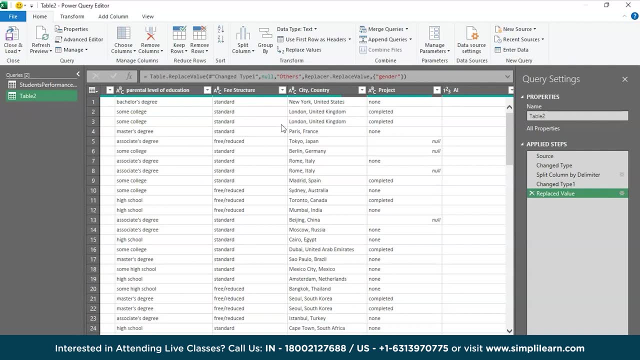 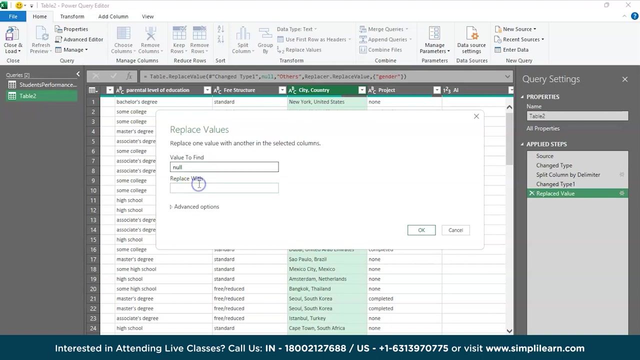 um, all the entries are of the students are from different cities, so it should be like they are taking the course in remote. that is the online course. now, wherever you find a null, that should be the students from the university as well, right, so again press as null in smaller case: university student or uh. yeah, you can write it as daily scholar. 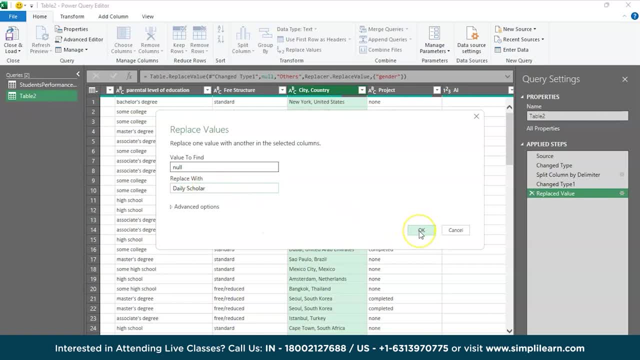 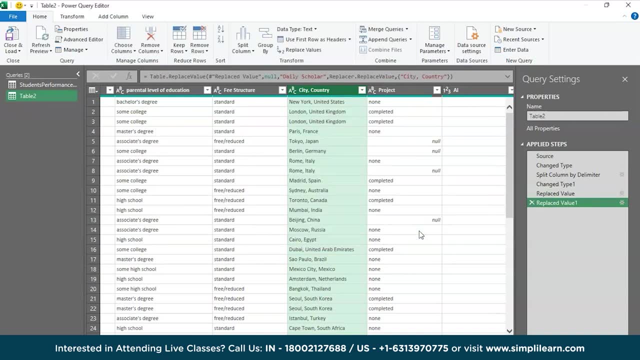 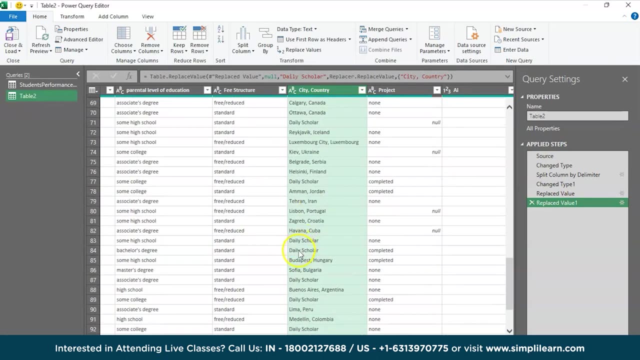 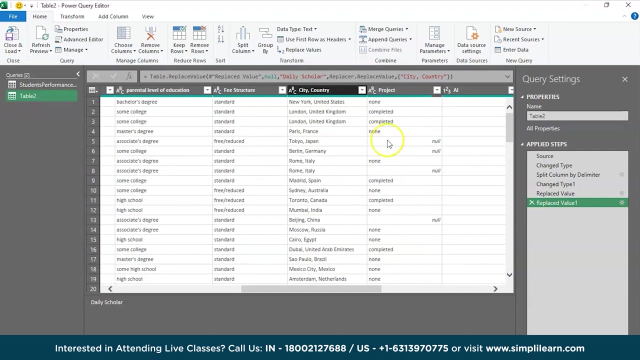 means this particular student is going to college every single day and the remaining ones are, uh, taking up the course through online. there you go, so we have daily scholars wherever we have null right. so that's it, and now coming to project. so here, in a few places we have completed and in a 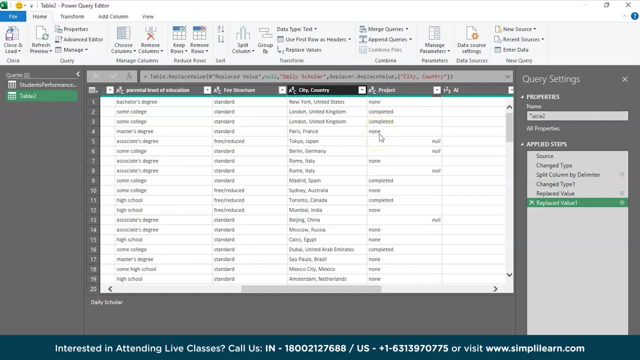 few places we have none, and in a few places we have null. wherever we have null, it is an indication that the project is still in progress, and in places where we have none, it means that that particular student does not have to do any projects or projects are not related to that particular course. it can be anything right, so let's try. 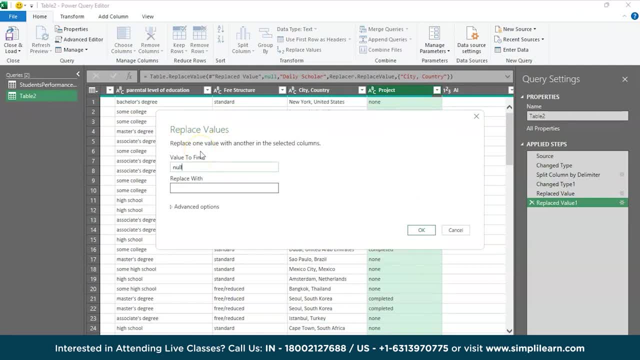 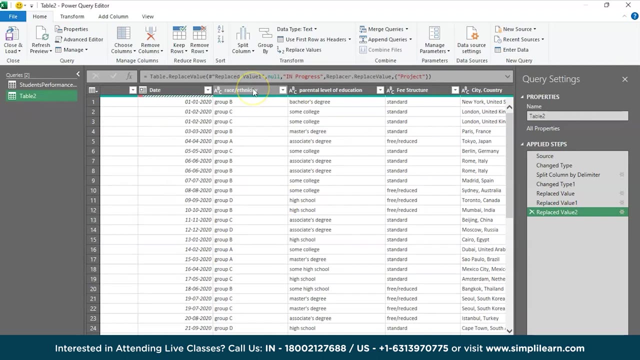 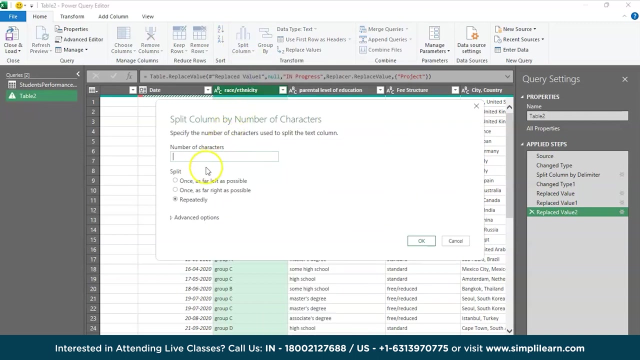 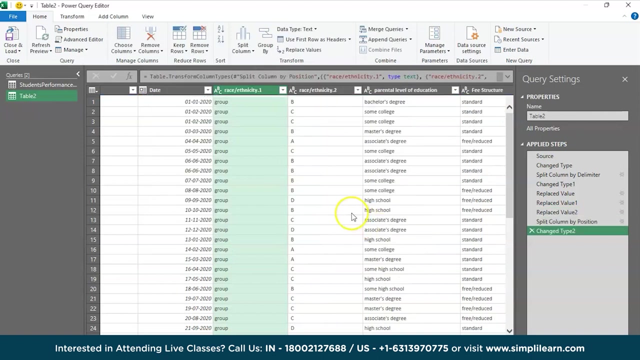 to replace the values. once again, wherever we have none, let's try to add it as: uh, in progress, okay, and let's say we also want to split the groups. so we can do that by split column by number of characters: g, r, o, u, p, five characters, right, so press ok. and now we have eliminated the first five characters and 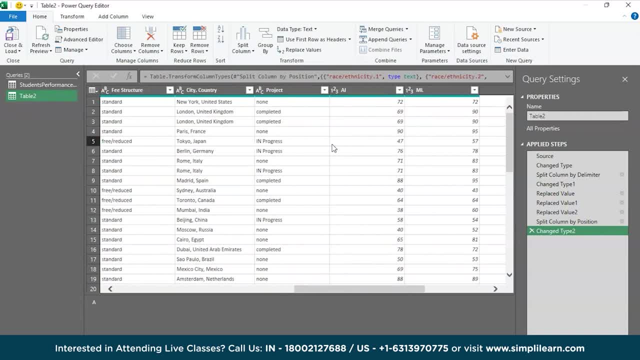 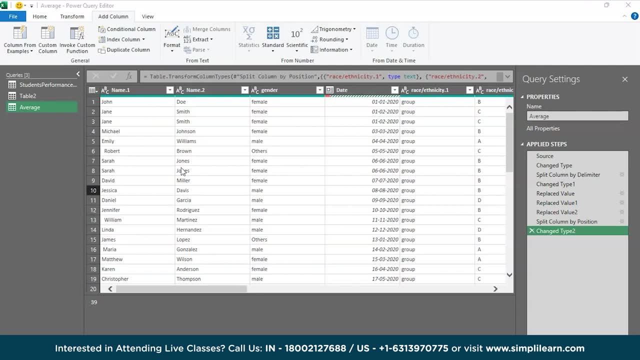 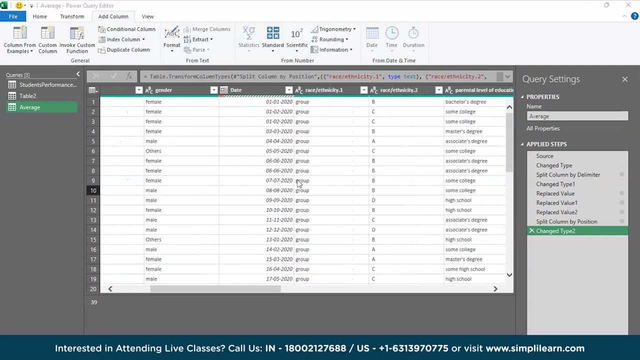 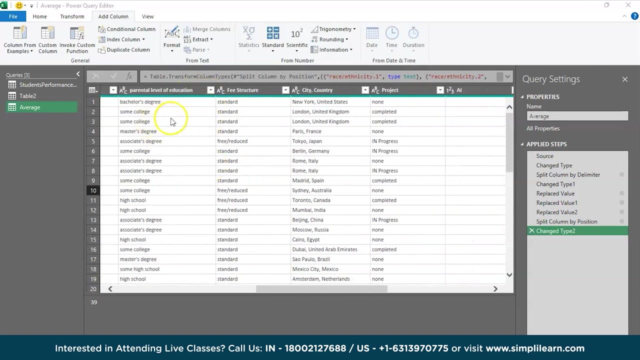 separated the group, right, so these are the groups which we needed now. so far, so good. the data is clean, so we have our first name and second name splitted, the gender column sorted, the date data type has been sorted so we have one single data type for all the dates and group has been separated. and uh, some college. so yeah again. 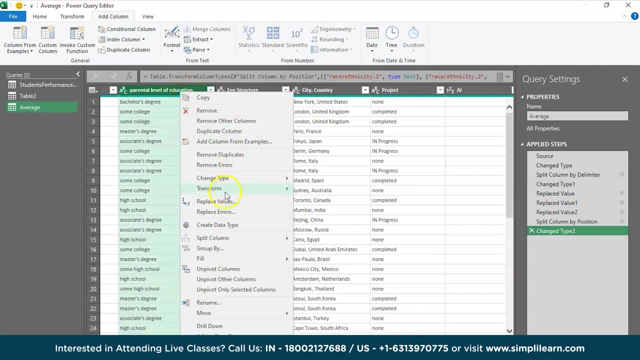 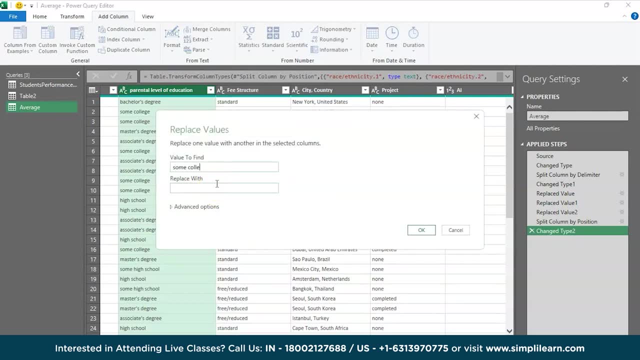 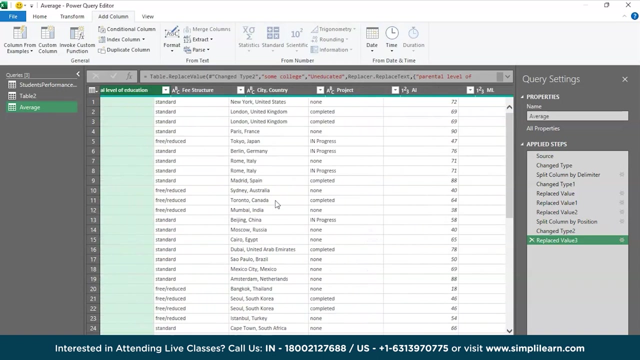 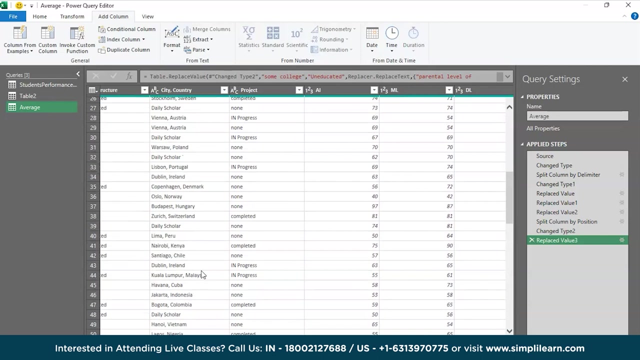 this particular column. if you want to change something, let's say, if you wanted to replace the values of some college to, you know, uneducated or something, something relevant which makes more sense, you can do that. so it's done as well. and the fee structure is also standard, and country, city are also done. so wherever we had no data, it's been recorded as a. 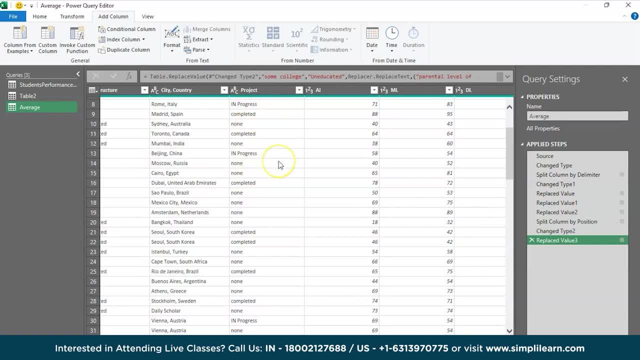 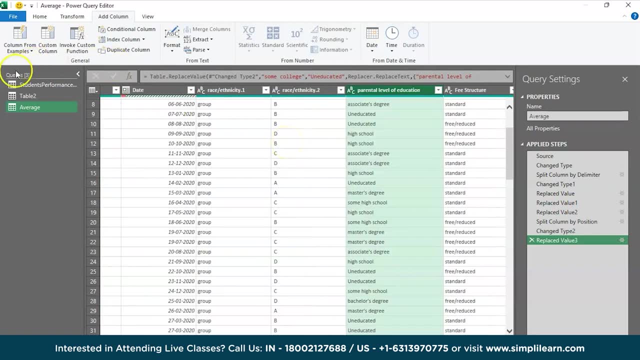 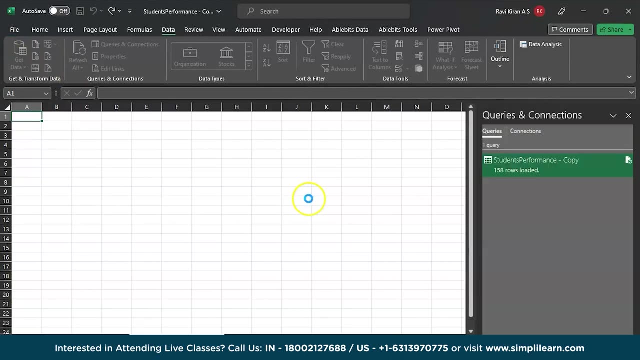 daily scholar and progress about the project is set and the marks achieved in AI MLDL. everything is sorted now that we have the cleaner data. all you can do is just click on the home button and you can choose the option close and load. right now you have the data loaded onto your excel spreadsheet. 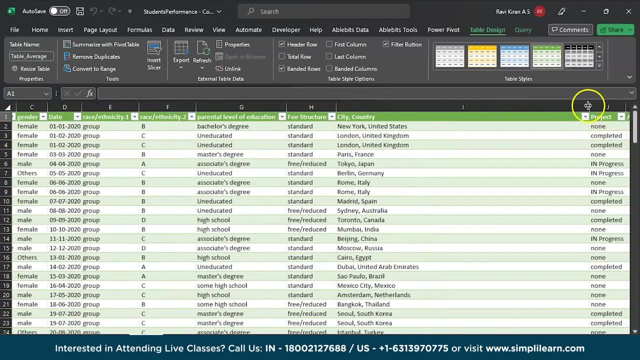 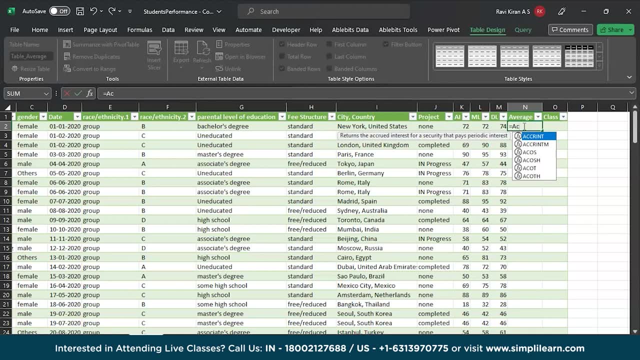 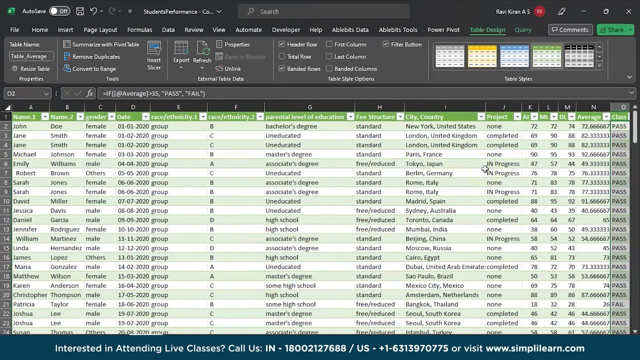 it's this and adjust the column width. now we can calculate the average. all the three rows. apply to all the rows and again your if condition. if this value is greater than 13 five, then student is has passed the test, else it's three. now you can apply the same to all the rows and done. now your data is clean. so 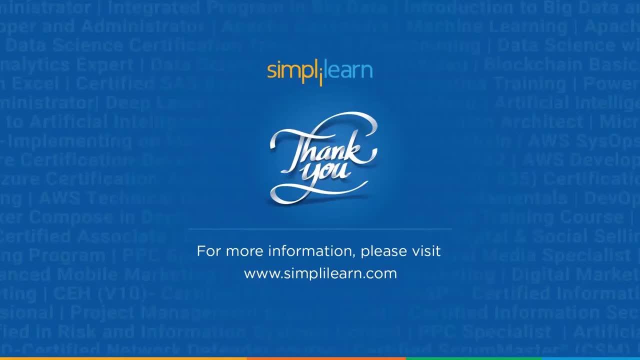 that's how you can do data cleaning in Excel. so if you have any queries regarding any of the topics covered in this session, or if you require the resources that we used in this session, then do let us know in the comment section below and our team of experts will be more than happy to resolve all.